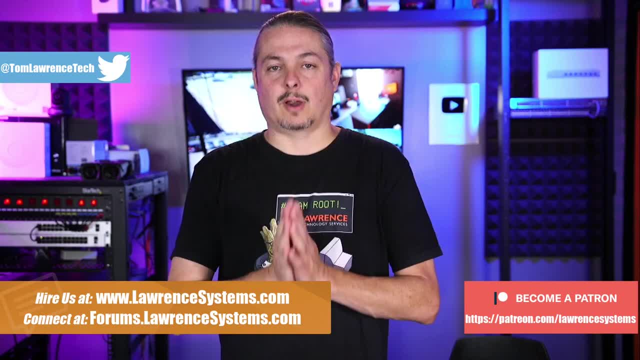 check out the affiliate links down below. They're in the description of all of our videos, including a link to our shirt store. We have a wide variety of shirts that we offer on this channel If you'd like to help keep this channel sponsored. 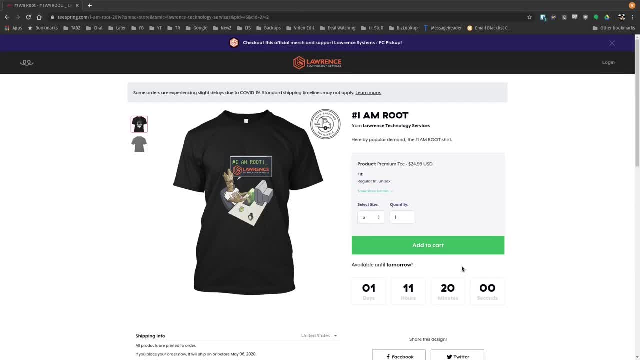 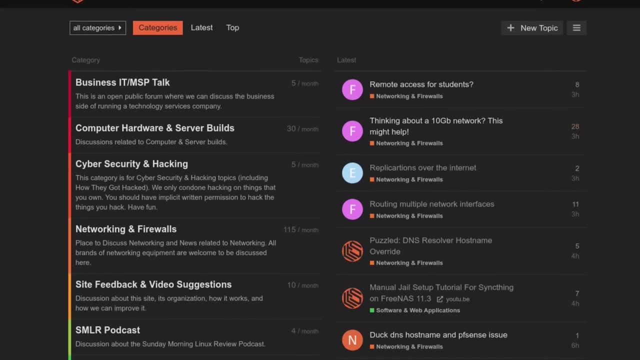 and new designs come out well randomly, so check back frequently. And finally, our forums. Forumslawrencesystemscom is where you can have a more in-depth discussion about this video and other tech topics you've seen on this channel. Now back to our content. 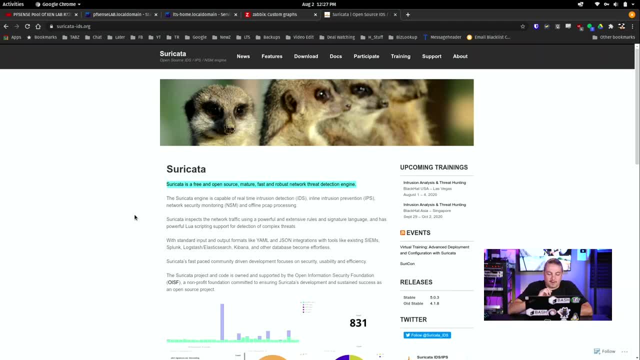 And we'll begin right here. Sericata is a free and open-source, mature, fast, robust network threat detection engine. That means it can look at the traffic coming in and detect threats, And a lot of people start assuming: oh, this is what I need to help secure my network. 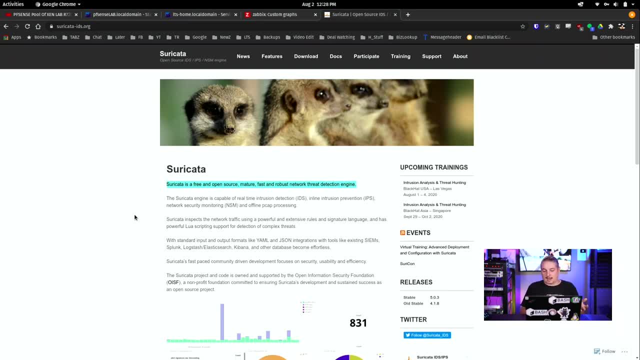 Well, it can only detect threats. And IDS versus IPS is intrusion detection system versus intrusion prevention system. And then, really, the difference is a checkbox, whether or not you want to block the threats it determines. And before you're wondering why you shouldn't just block everything that it detects, well, false positives. False positives are what. 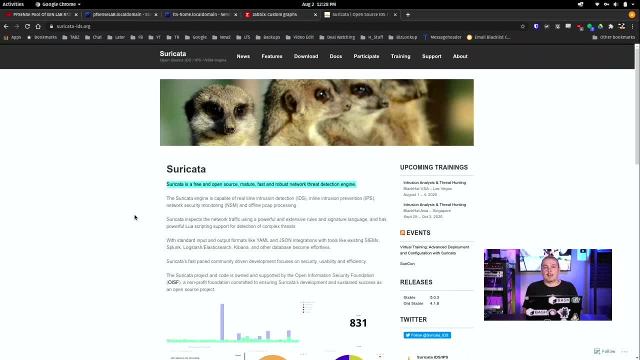 we're going to talk about. We're going to talk about how to tune the rules on this and how to set it up, But beware that this is not a one and done type of process. Occasionally you'll have to go back and find the things that got blocked accidentally. 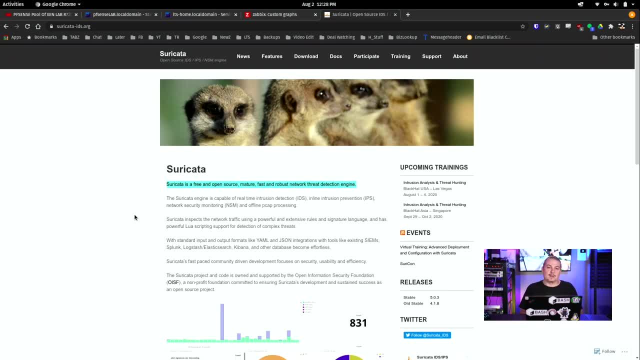 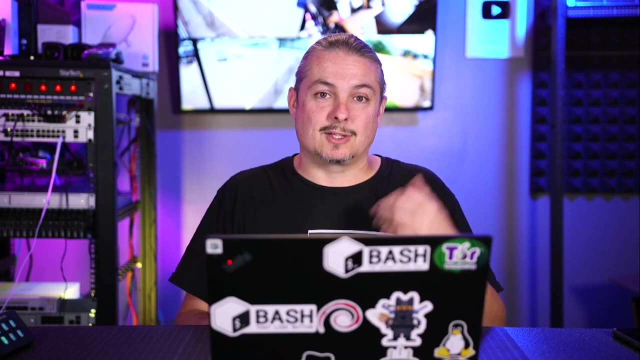 This is just part of doing intrusion detection, And a lot of the reason for this is because the tools are becoming more and more blind to the traffic. As traffic becomes more encrypted, there's less information for it to use to figure out exactly what that traffic is. So this is where 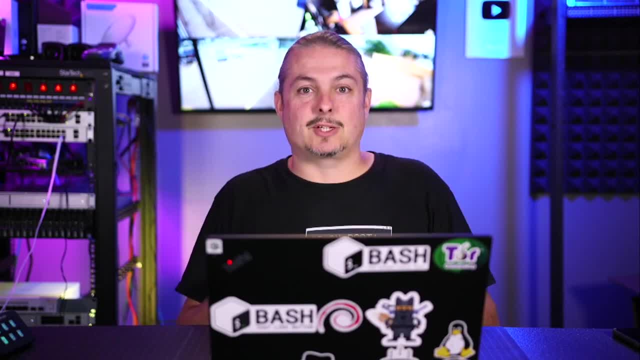 false positives come in quite a bit, So an encrypted piece of traffic happens to match the pattern of some of the threats that it detects, And that's why it's so important to have false positives. So let's take a look at some of the things that we've done in the past. 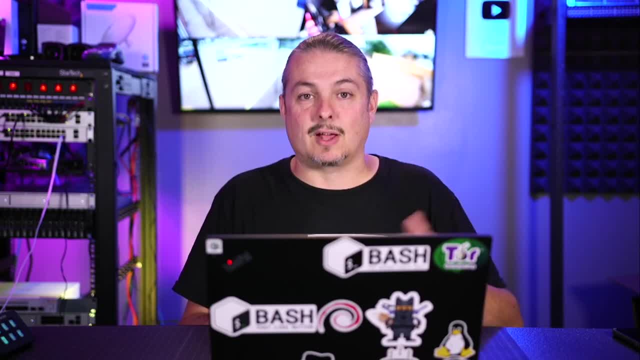 And they do their best not to have false positives, but we've run into this ourselves. We've had things that are custom, like some of the remote support tools we use, that are running on a non-standard port And Sericata will flag it and block it going. 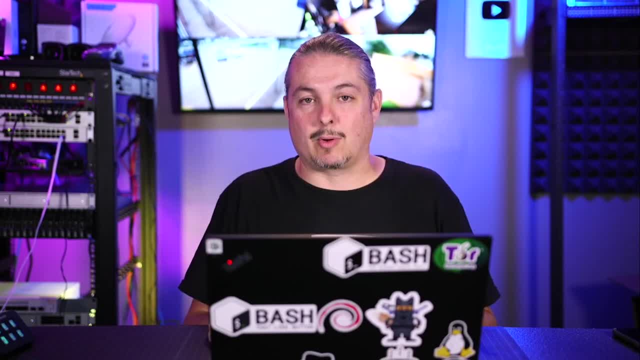 I think that is this attack And right away I can rule those out. going well, I'm not even running that software on here And we also figure out ways we can repeat it by going well. it looks like every time we open up this remote support tool and do a file transfer inside. 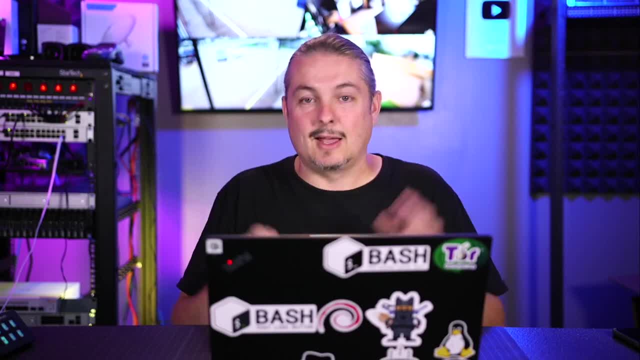 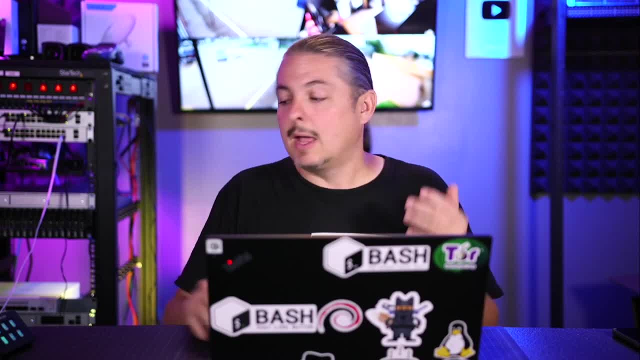 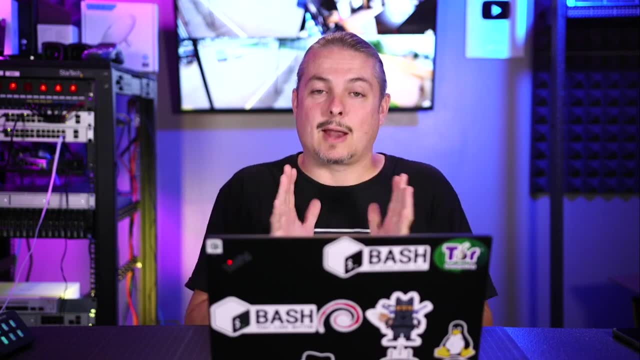 that's where we're going to cover how to set it up and how to get these rules tuned. But I just want to preface all this before you go any further. This is not a check the box, and it just works and makes your network more secure. Now the other side of Sericata, where it's much more effective. 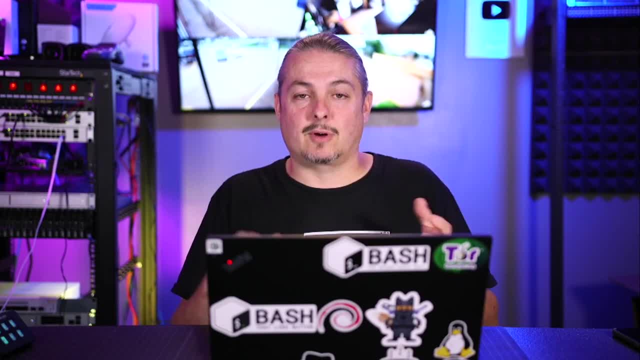 versus less effective is going to be if you have services you're running and you have ports open. So I'm running a web server, for example, or I'm running a WordPress site and I want to put my firewall with some Sericata rules in front of it. Sericata is quite good at detecting some of the 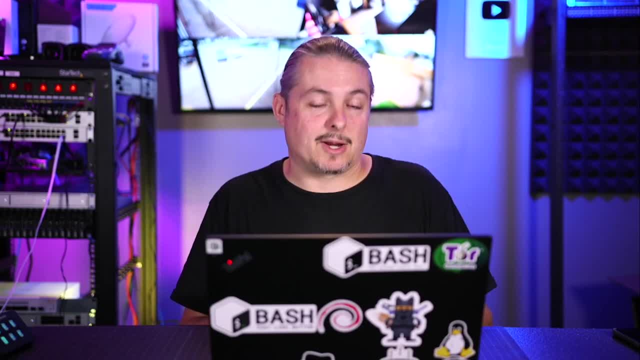 inbound potential problems that are coming in and pattern matching those because you have ports open. If you're just a home user, the limited amount of success you're going to have is because a lot of these devices on your network like your IoT network. they reach out through whichever. 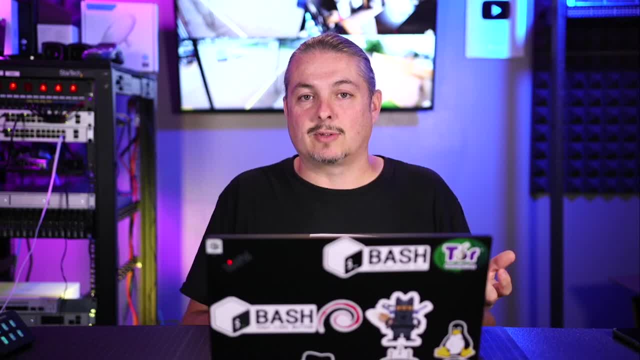 protocols to get their data they need from whatever cloud servers they want to talk to. That's not something provided unless it was not encrypted. It's not something Sericata is going to have an easy time deciphering what it is And you'll probably just get a bunch of false. 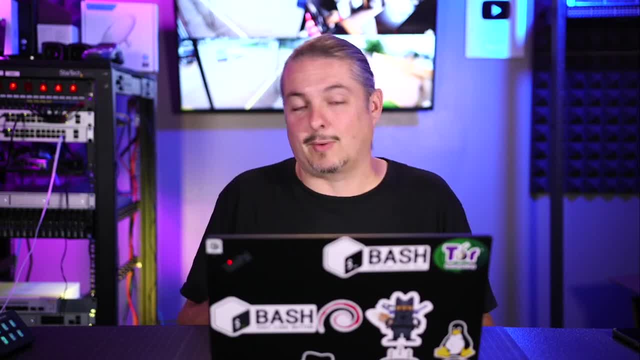 positives and spend a lot of time doing it. Either way, I think it's fun and it's a great learning process to do that. But, like I said, I just want to preface this video with those caveats, because that's something I did not do very well in my last video And it is probably 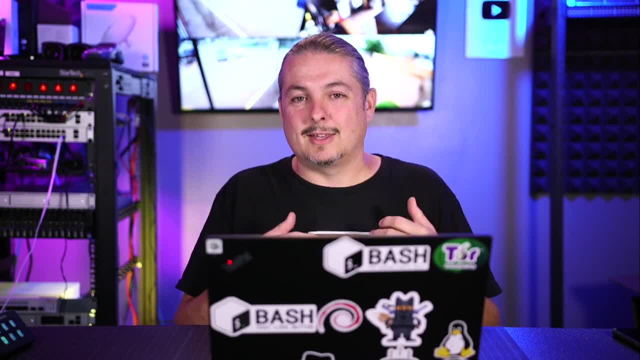 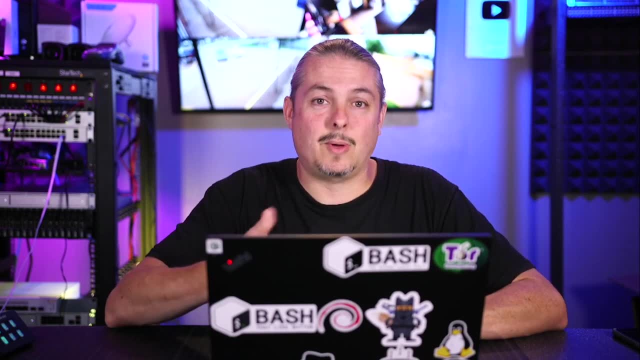 the number one question that people contact us about is: can I just set these and it fixes all these problems and makes my IoT safer. No, not really, But I do have an active network and we're going to show what false positives show up on a default install, So let's get started on that. 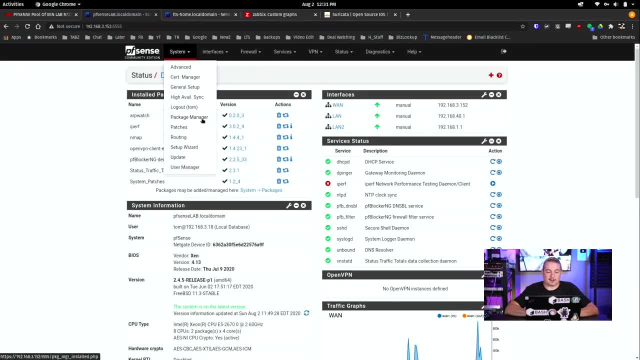 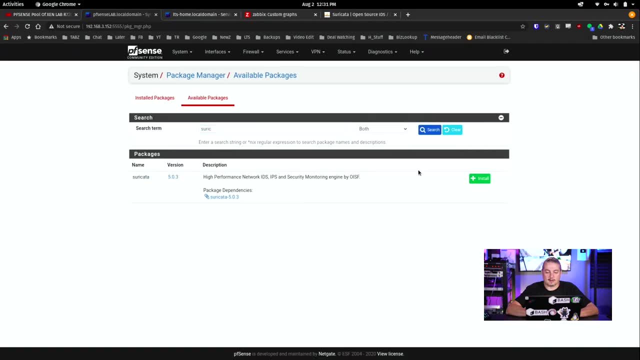 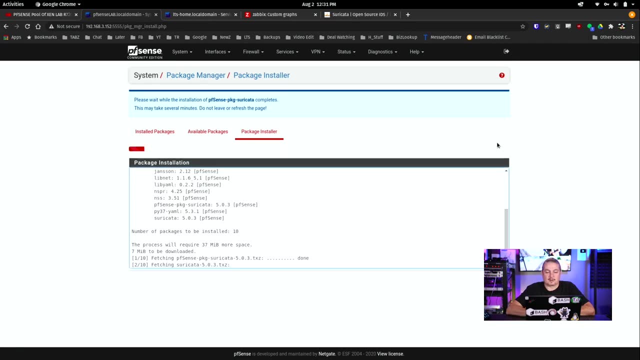 And install the plugin first. So we go over here to Package Manager: Available Packages- Sericata Install Confirm. So after this is installed, we're going to go through how to set up the rules. This is the important part, for the rule setup is getting the downloads proper, Because the defaults right now. 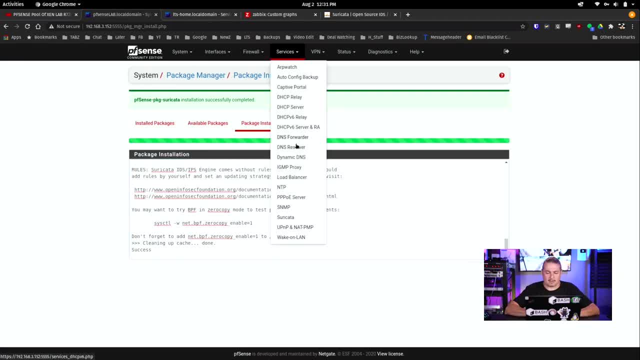 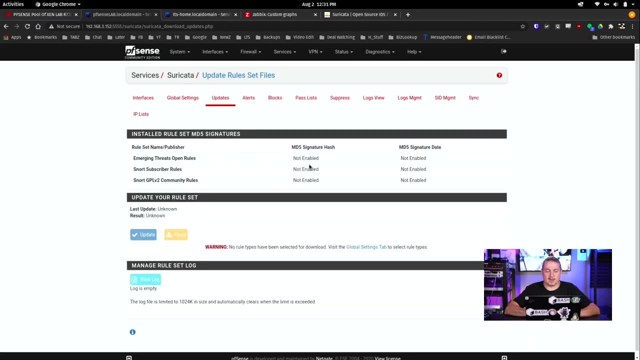 and I don't know if this was true back when I did the other video, but right now the default downloads don't work. So we'll go in here and we're going to go over to Updates And right here, we have nothing in here yet, And what these are is the rules and 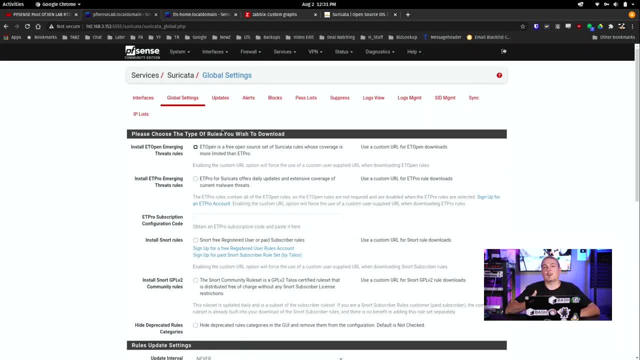 signatures And you can get a snort key if you want. I'm not going to do that for this particular video. We're just going to use the ET Open rules. So we have the ET Open rules. This is the snort free register. If you want to store those, we're going to do these ones here And I guess we can. 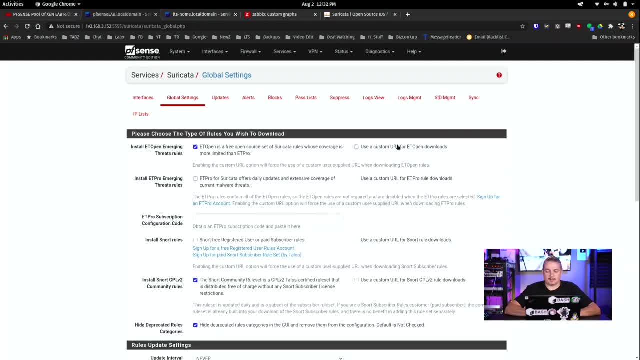 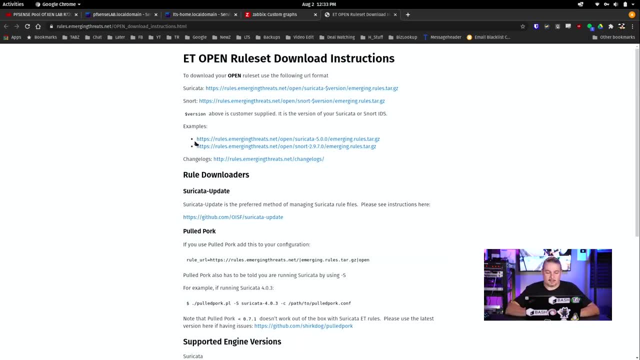 hide the deprecated rules if we're not using it, But we do need a custom URL. Now here is the emerging threat free rule set that you can get, And the good news is, as of right now here in August of 2020, this rule set works fine because 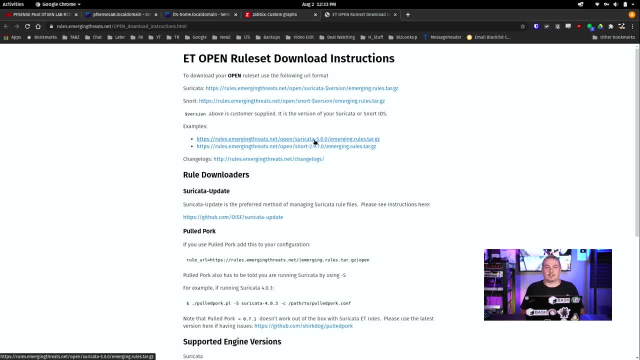 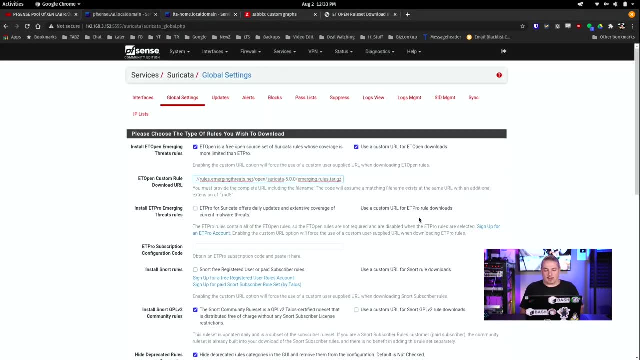 it's the 5.0 rules. Sericata, inside of PFSense is running version 5.. So we're just going to copy this link. go over to our lab. paste in the custom download URL Now in the future, if you're using. 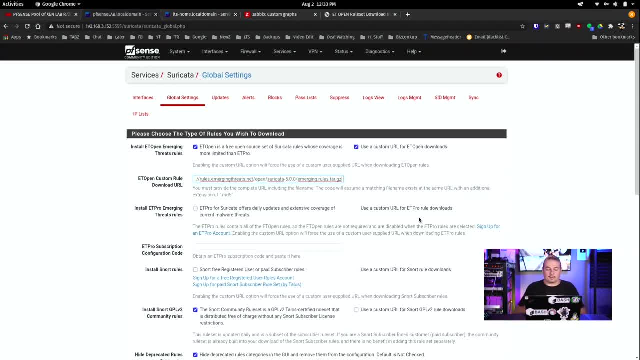 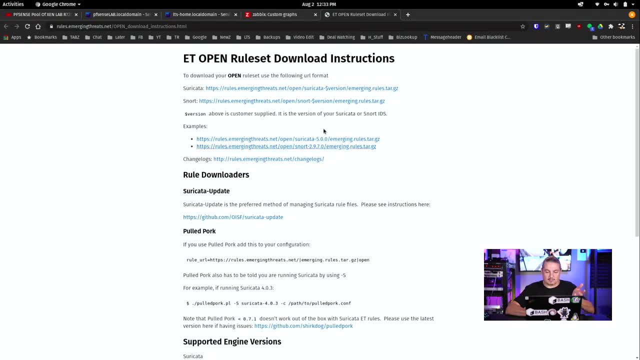 a different version. you want to match the version of Sericata with the version that you're doing here. So, because we're using the 5 series, I put the 5.0 in here. If you were running some old version. you kind of get the idea from here that you can switch versions. 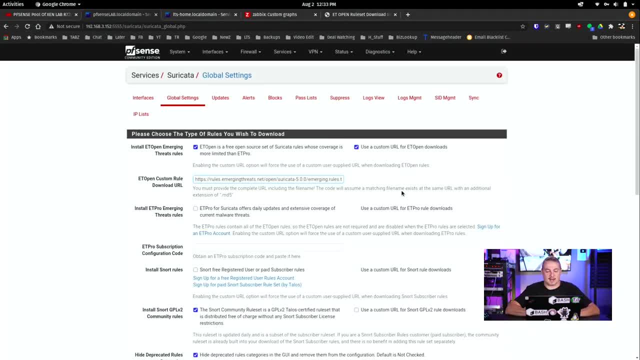 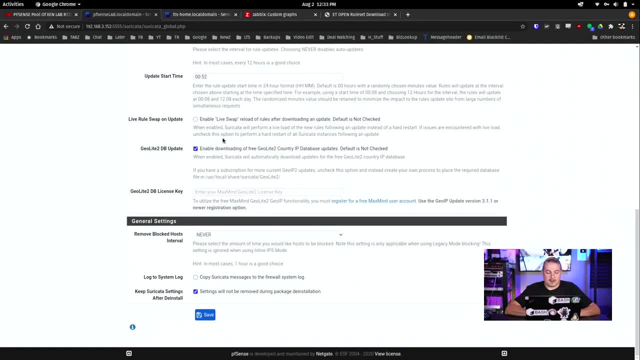 That's important that you put that in there, because the default one it tries to download doesn't work, So we'll throw in that custom URL, go down here and hit save. Now, down here at the bottom, I'll mention: this is the blocking. It is up to you when it blocks. 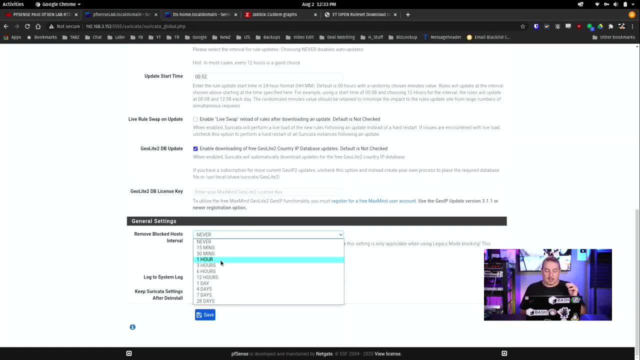 something. if you choose to turn on the blocking, not just monitoring long before those expire, One hour is not a bad idea. If you say never, you'll end up with things in a block list and you may have sites that get blocked. You may end up having them blocked. 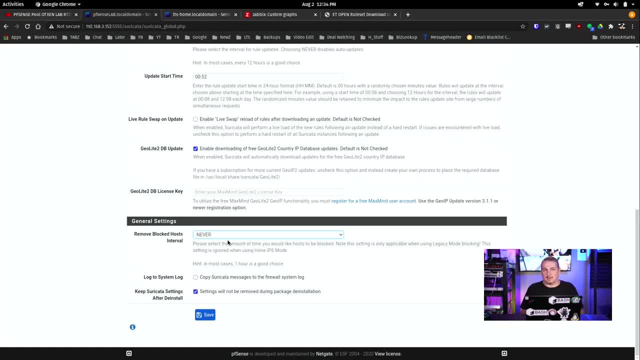 permanently. We'll cover how things get blocked and how you can eliminate things in the block list, but it's at least let them expire. If you don't let them expire, sometimes I find at least trouble. So that's kind of just some housekeeping cleanup, If you wanted to say four days. 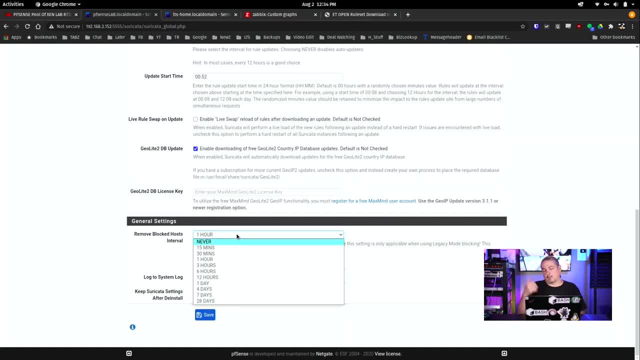 that way, if someone scans you, trips the trigger. that would cause a block. that person then, for some amount of time, would not be able to do it again. It's usually a bot anyways, but you'll end up with a lot of these and it'll fill that up pretty quickly of all the blocks it starts putting in. 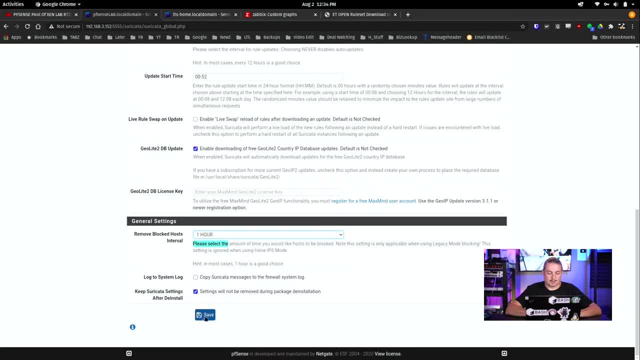 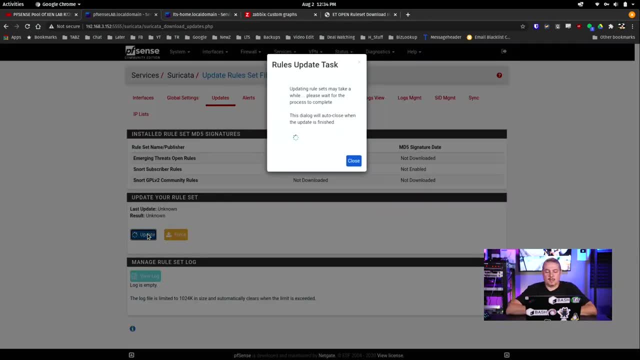 there, just depending on how involved you get with the rule sets. So we're going to go ahead and just set it to one hour. All right, now let's go over here to update. Let's update the rules, And this is pretty quick task, goes down, grabs those rules that we put on there. If you had. 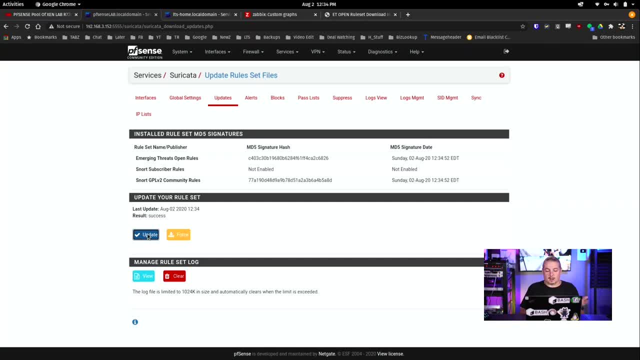 those snort subscriber rules, which is something you can sign up for. you'll get those. So now we want to make sure to hash and cool. Here's the rules updated and in there Now, when you're doing these rule updates as well, it's got a timer so you can set how frequently you want these rules. 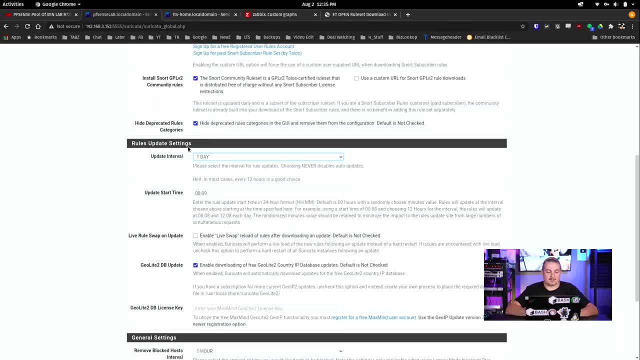 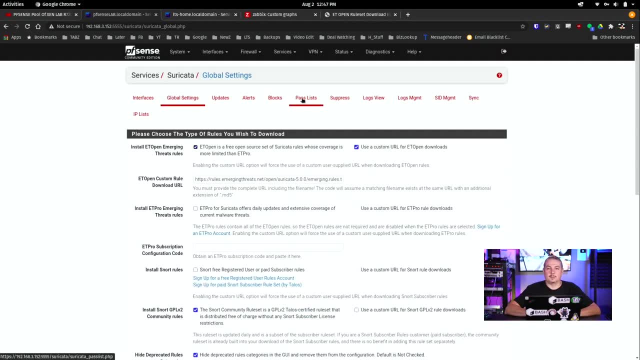 to update. I would say once a day is probably fine on here. That's under the rule settings. So we have that the rule settings for one day, and maybe set this to one hour. So we'll just leave it like that, All right. next we have to set up the interfaces, So we'll go over here. 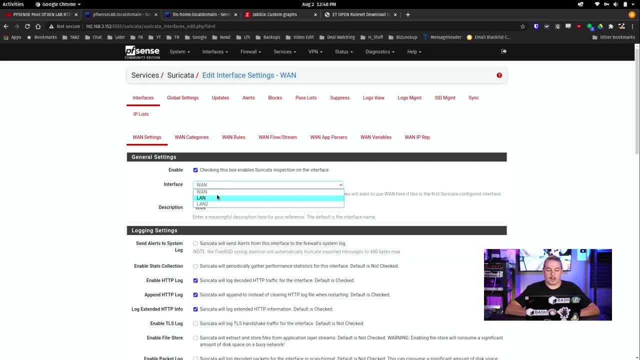 interfaces and we're going to add our first interface Defaults to WAN. if you want to put WAN, you're going to get a lot of noise And by default PFSense out of the box is going to block all incoming ports. So if you put this on WAN, all the ports are blocked but it's still going. 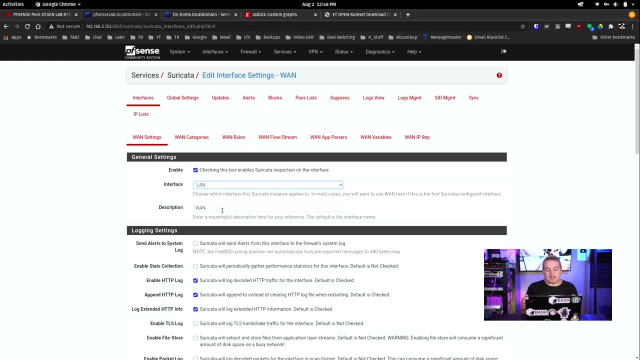 to sense all the noise of all the things that hit those blocked ports. So it's up to you if you want to put it on there. It's going to definitely take up some CPU cycles. It's definitely going to create some false positives because it's just well, not really relevant because someone's 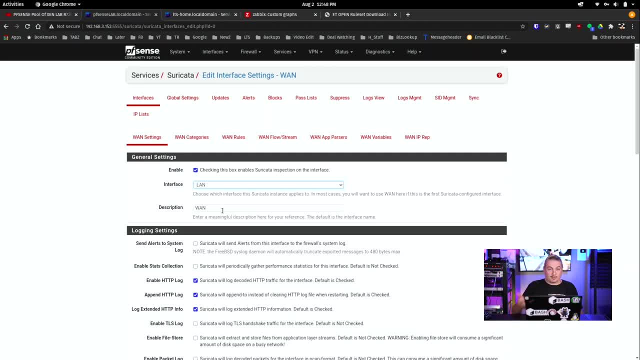 scanning a port that's not even open makes for a lot of logs but doesn't necessarily make for much actionable intelligence, other than some people panic and go, wow, there's this much going on on the internet? Yes, there is, So we're going to put it on the LAN side Now for each interface. 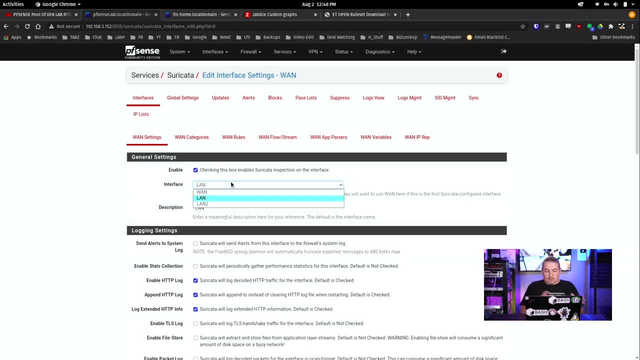 you want to create a different rule category, or maybe you don't. this is up to you. And my example here: LAN would be just normal LAN traffic And maybe we want all the rules applied to that. But let's say our guest network. we don't necessarily need blocking turned on for 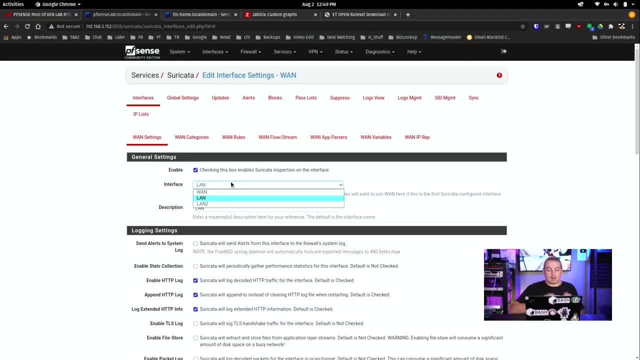 our guest network, but we're maybe curious about what things are going to happen. So we're going on in that network. So, a guest network: maybe you turn all the rules on but don't turn on any blocking. Now, these are different things you may want to do on a per interface basis, But once you 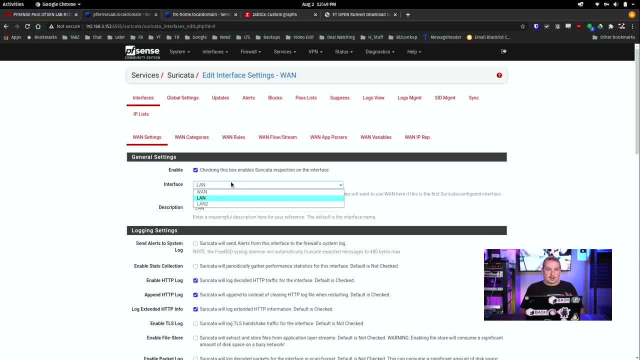 configure an interface. you can also clone those rules on there. We're going to cover both how that works. So it's kind of up to you on how you want to do that. If you want to just enable all the rules for every interface or maybe have a less restrictive policy on your LAN and a more 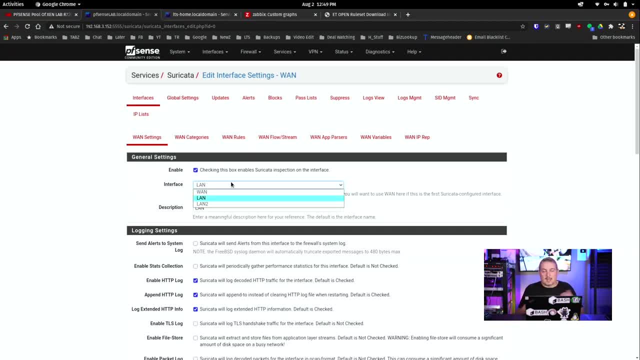 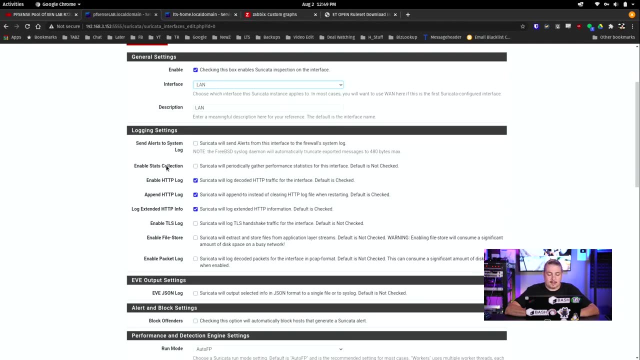 restrictive policy on maybe a specific secure network for your servers. Like I said, there's a couple of different options For this demo. we're just going to enable all the rules to make it quick and easy. So LAN: LAN send alerts to the system. log- not necessary, but you can do that. Enable stats collection You. 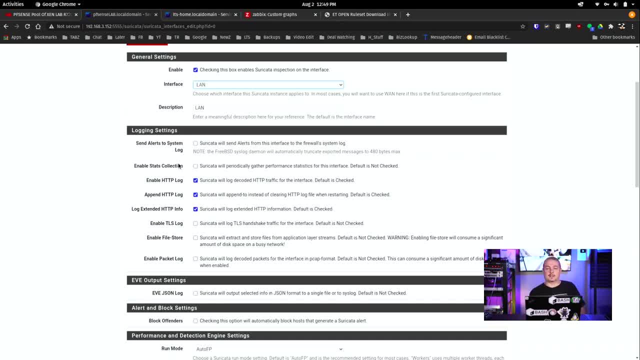 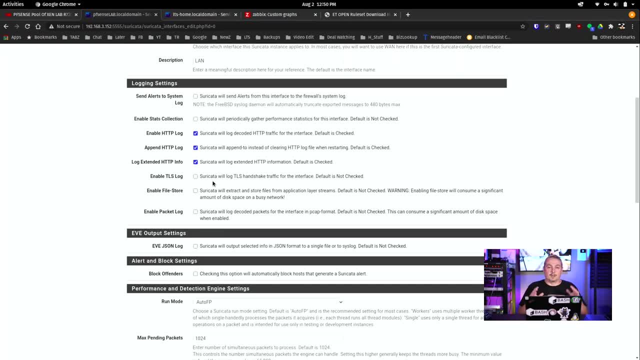 don't get any pretty graphs for the stats collection. It just logs some of the statistics and puts them into a log file. in case those are interesting to you, You can have those. Enable TLS log. Now remember, intrusion detection systems like Sericata are blind. 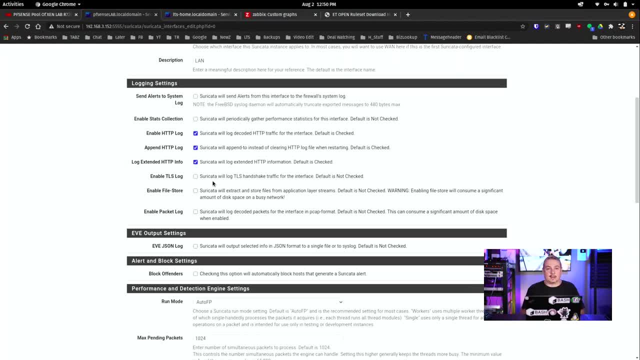 to the majority of the traffic that's encrypted, but it can at least log that a TLS connection was made. Maybe you need that, maybe you don't. It is also blind to files that were transported via encrypted TLS connections. but if they are not transported, 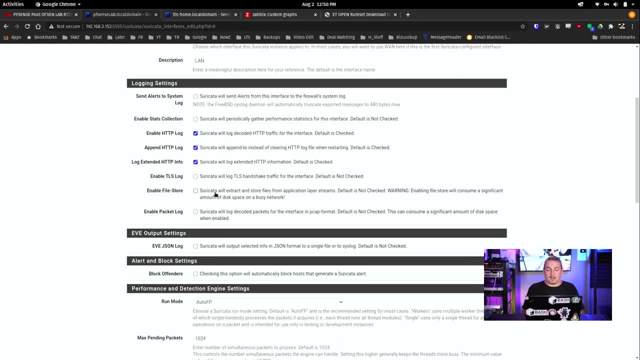 that way you can enable file store. Make sure you have a PFSense system with enough space if this is something you'd like to do, And the same thing with packet logging. You can do full PCAPs on these, but you have to have somewhere to put them. So make sure there's plenty of space. if 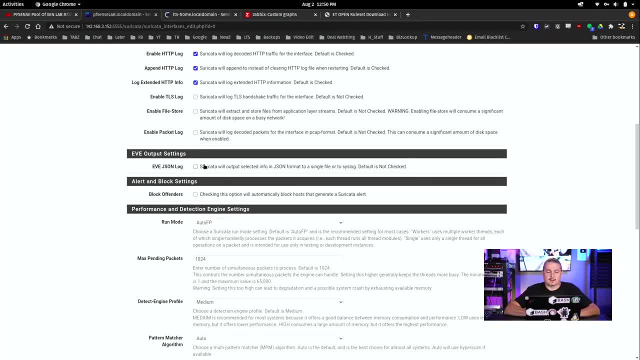 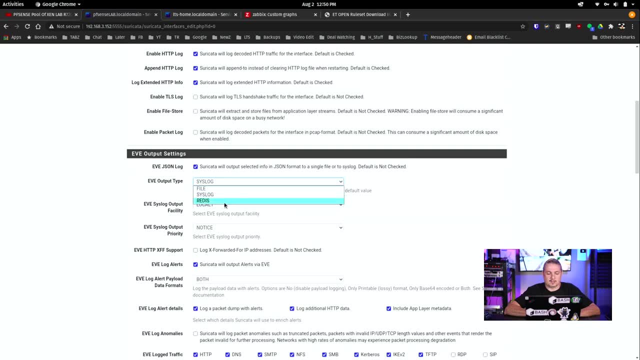 you choose to do that, EVE JSON log Sericata will output selected logs, but you don't have to do that. You can also export the logs in JSON format And actually this opens up quite a few options, including sending them to a Syslog server, a Redis server. This is a methodology, so you can. 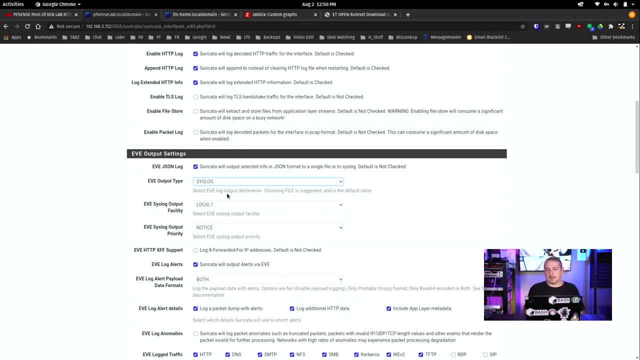 export all the logs to something else for log parsing and further analysis, Maybe a different SIM stack that you have like a security system that does some analysis and all the generated data. That's what that option's for. We're not going to be using it. It goes out of scope with this. 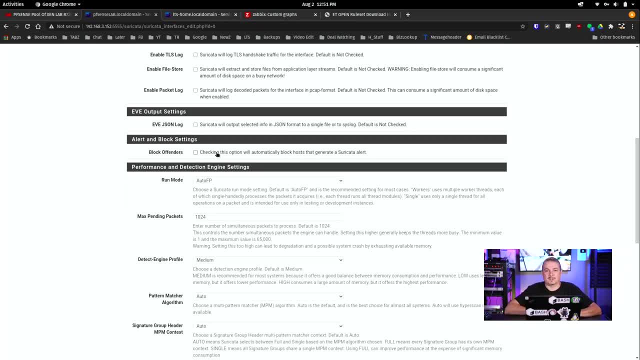 This. I do not recommend checking when you are first setting this up, because when this box does, it starts blocking the things it finds You first set this up. I recommend leaving this off and going back and turning it on And when we show you how you tune the rules, you go through the. 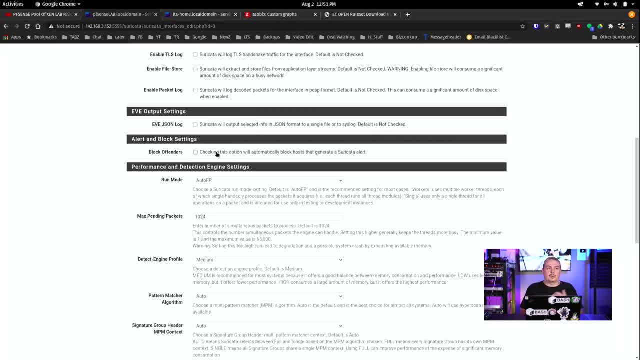 tuning for at least maybe a week of usage. Tune the rules. If not, you'll end up being blocked constantly and then forcing yourself to tune the rules- A less pleasant experience. but it's up to you the method you want to follow. For me, leaving this off for the first week you set up Sericata. 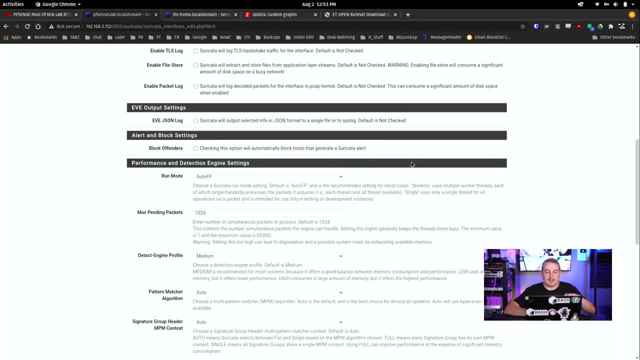 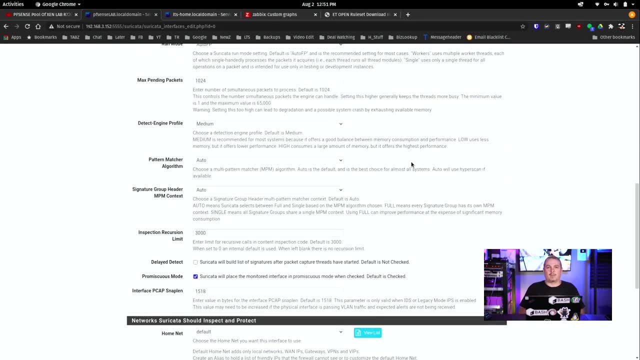 while you enhance all the rules probably makes the most sense. We'll leave all these at default. There's some edge cases and I believe I've talked about them on my Sericata transparent firewall video. You can find it on here for your Sericata transparent PF sense. It's really cool. 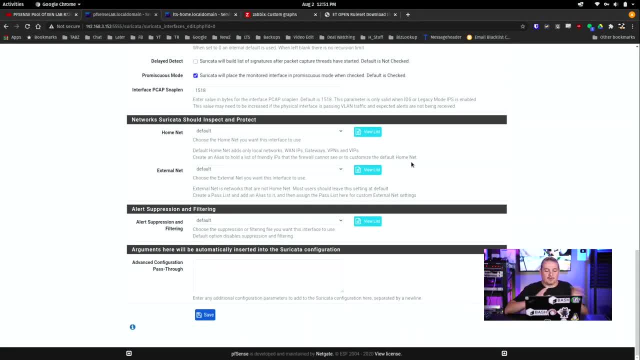 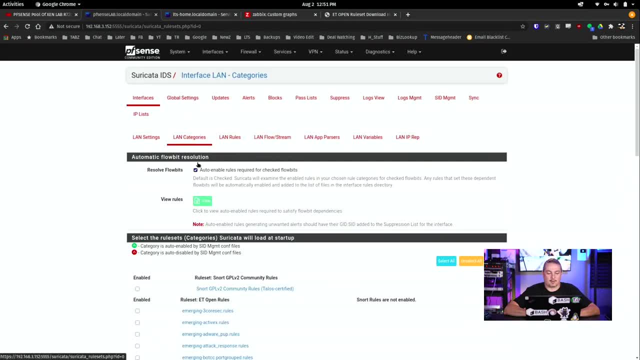 It works. There are some special tuning parameters from those, but for the rest of it, no, we're just going to leave everything else at default and hit save. So we create the interface on here. Categories: We're just going to do select all Now based on the global settings and what rules. 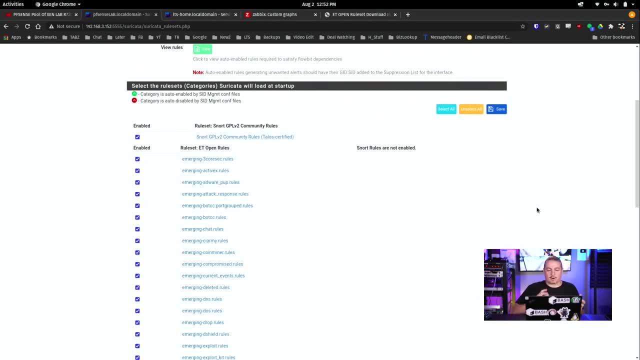 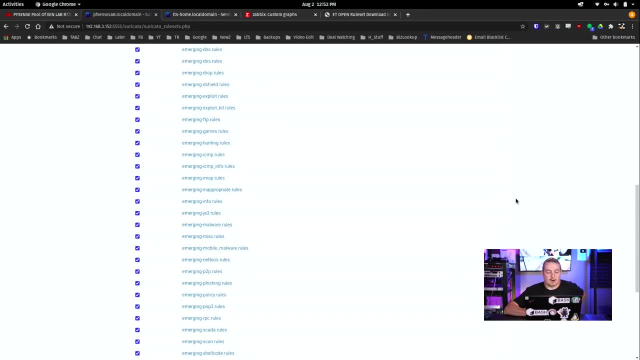 you pulled in there- which we did- the Emerging threat rules and the snort GPL rules. You can go further and get the paid snort rules if you want, and it will make more rules that show up here And I checked the box on all of them. 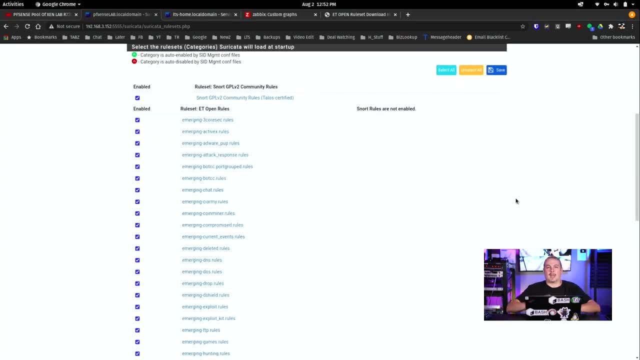 but warning: by doing this I now have the most potential for false positives. So what happens is the more rules that you check, you have to think about the rules that really matter to you, And this is when you're thinking back, like I said, about which rules apply to. which interfaces Selecting all on all interfaces creates the most amount of work for you. so you're going to do the rule tuning, but doing it on a per interface basis where, like I said, if you had a server network and you go, this is one I want- really watched further and better. 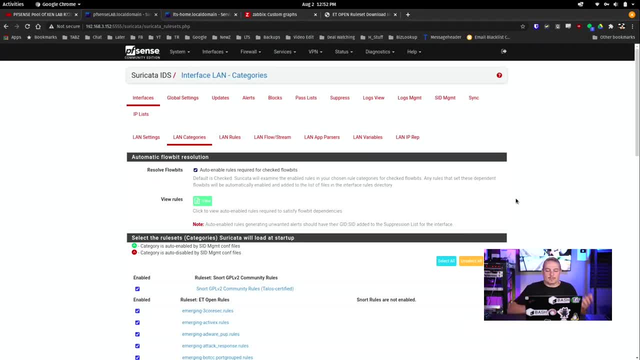 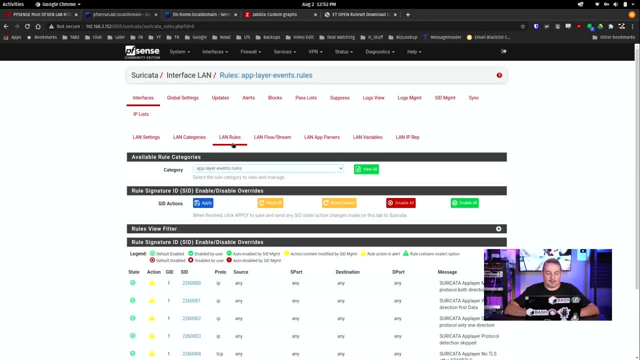 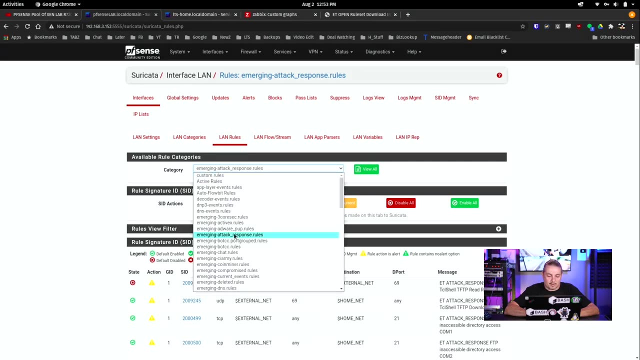 versus my guest network, which I don't need that many rules, But, like I said, these are some of the fine tuning that you can get in there, So we're going to hit save on this. Then we have our LAN rules over here, and these are just the details of those rules, So let me find one that's got. 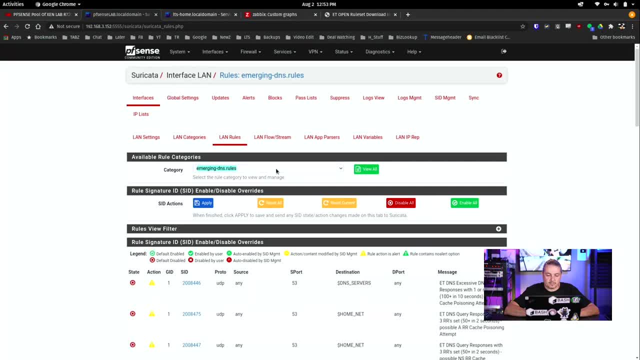 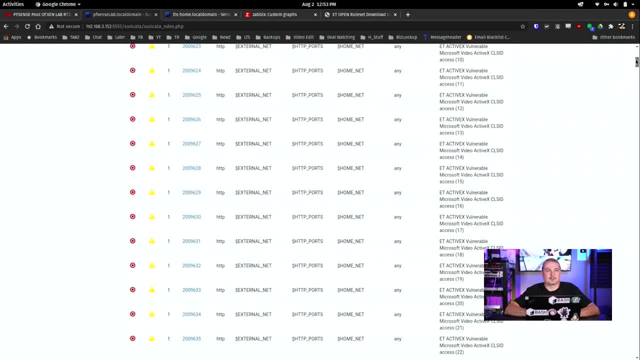 probably a lot. Maybe the NS rules, bot rules, ActiveX rules, quite a few ActiveX ones it tries to look for here, And what these are is the individuals. So you have the categories on the other page. These are a. 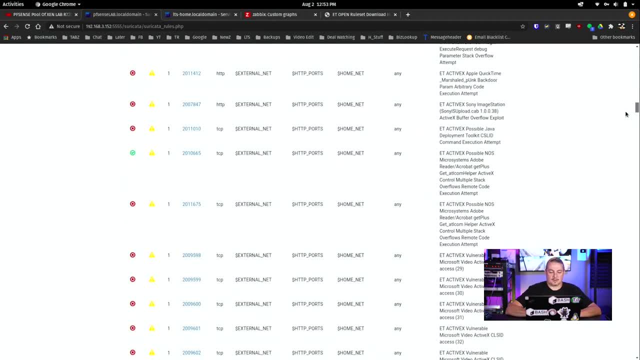 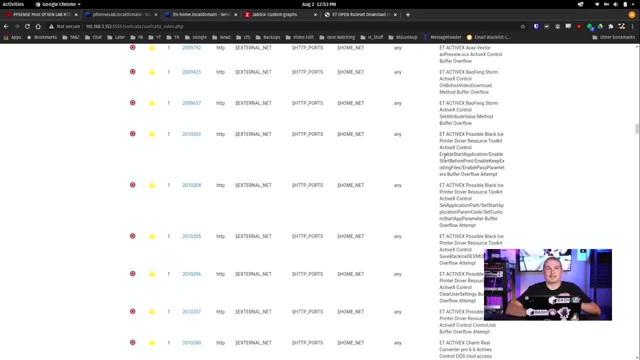 breakdown of all the details in those categories. So this is going to be what's enabled and what's disabled And they have some notes inside of here possible Black Ice printer device resource toolkit. but some of the reasons these are disabled by default, even though we checked them. 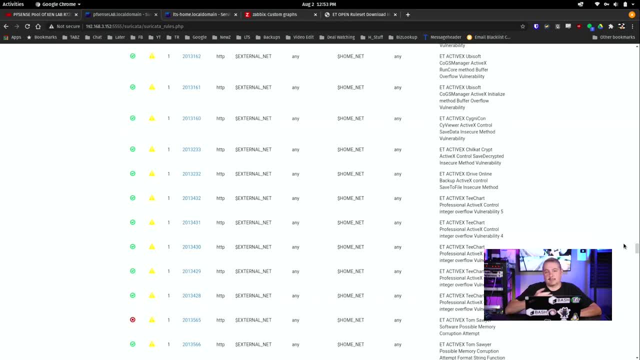 and you see those rules are disabled by default. So you can see that these are disabled by default. And then this one right here is the one you always see the red X's. that's because of the number of false positives they have. So they know that rule exists, but they also don't enable it by default And it 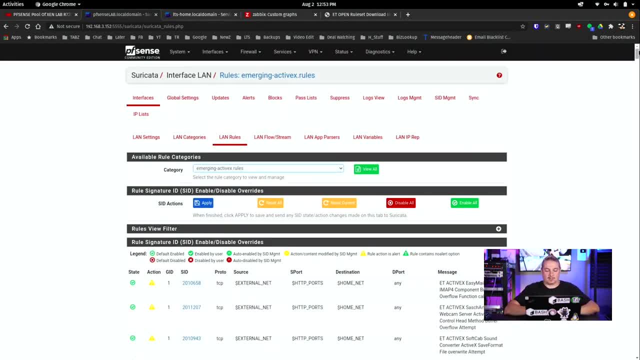 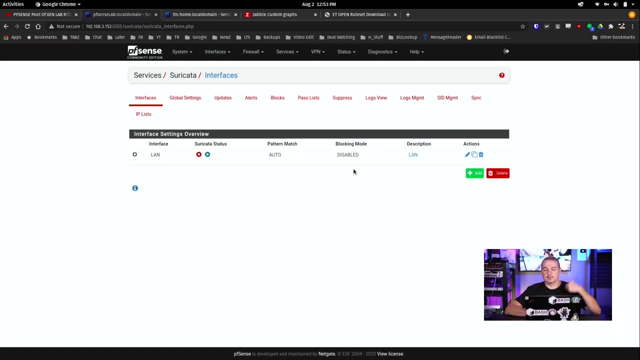 is up to you if you want to decide which rules to or not to tune on there. So that's pretty much it And we go back over here to interfaces. And if we wanted to duplicate this same rule set to another interface, once you have it set up and we're ready to go, you can just go. 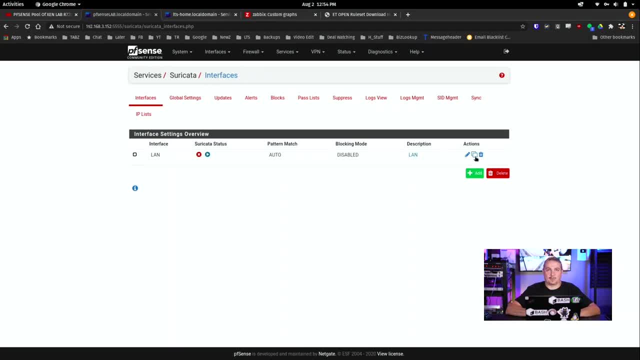 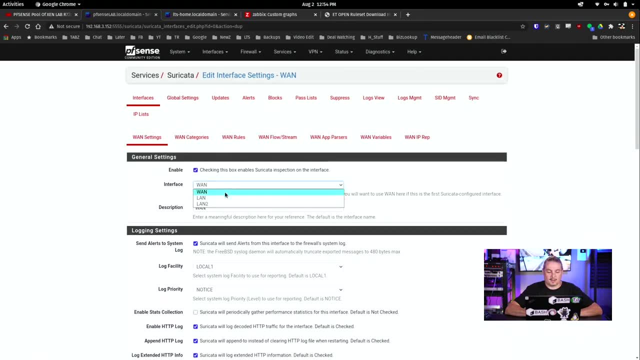 to this little clone button here or add, so I can add another interface and go through the setup again. But once you have- maybe you spent some timearta doing it or you had believe you are doing this some time tuning one of those interfaces- you can also just clone and choose lan2. 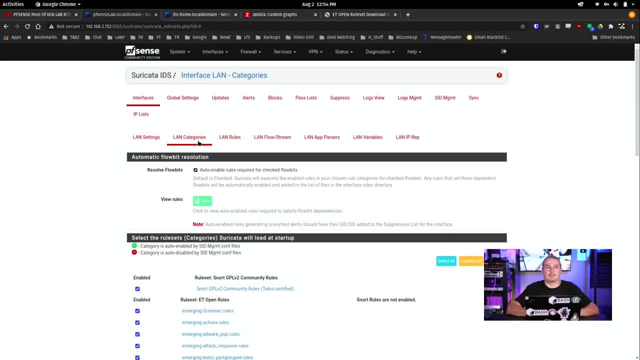 and already is selected for me. all the same rules. so that's the way you can easily, especially if you have like five diff interfaces, spend time tuning one of them, get it all set up how you want, then go ahead and clone that once it's all tuned. now, once that part's done, we're not going. 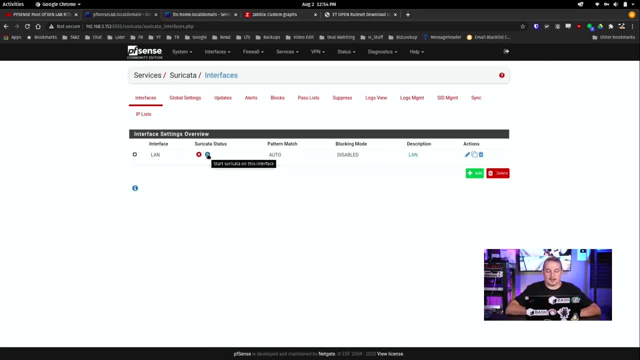 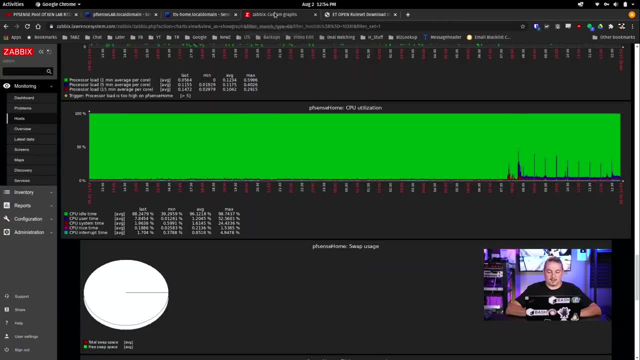 to save the second interface. you just click on the little start and it starts sericata on this interface. now we're going to get over to the fun part, the rule tuning. now one thing of note, and i just loaded sericata's. i don't usually run it at home and i just loaded it up on my system. this: 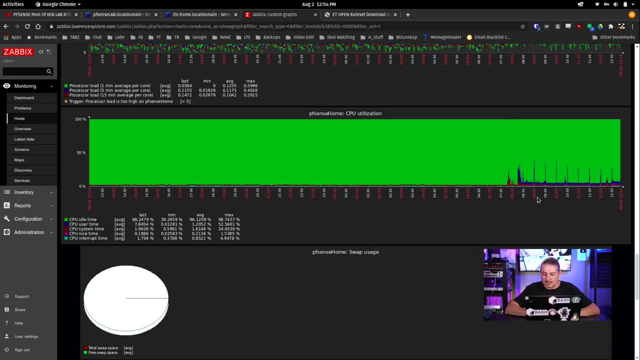 morning in lieu of this demo, and so i turned it on about- uh, this looks like about 8: 30 in the morning, so these little marks right here are when it started you can see how little firewall usage there was and how much more now. this is sg3100 neck 8 device. this is kind of the minimum i'd. 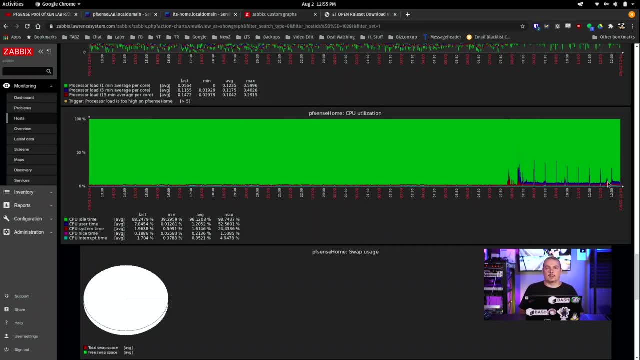 recommend um that you have in order to run sericata. now it is working fine at my house and it's able to handle this without much of a problem, but i just have a handful of devices and the kids are probably watching netflix right now and playing some video games. it's something that you have to. 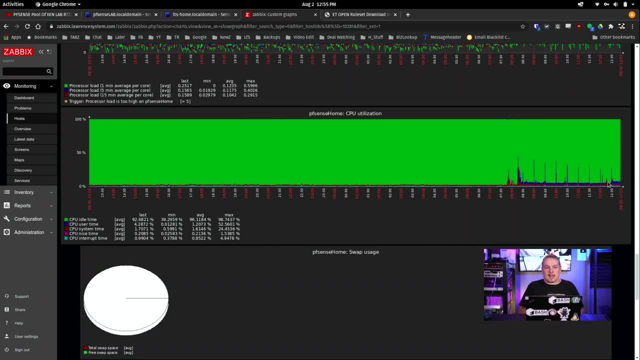 think about when it comes to scaling in here is: yes, it can handle it on like an sg3100 neck 8 device, but if you really start turning a lot of rules on and use it over time and there's a lot of connections on your network, you may want to think of upping that a little bit. but you can see. 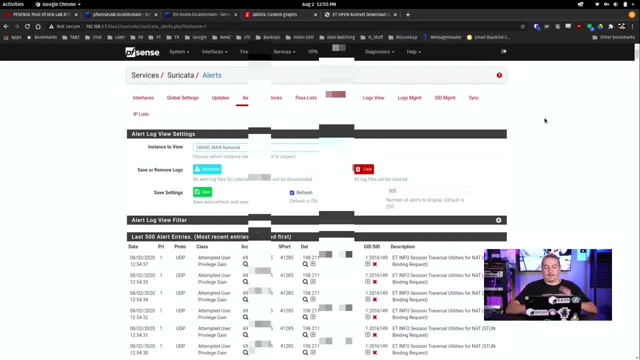 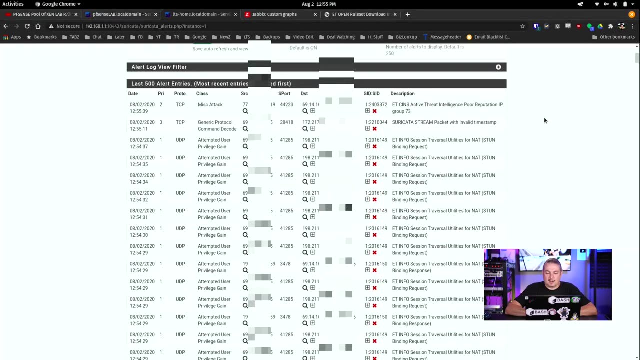 cost of cpu cycles right away. now i'm going to be redacting a lot of this because there's going to be so many um ip address in here, so that's why those are blurred out. so what we have here is the wan network, and this is why i said where you get a whole lot of things on here. now i happen to 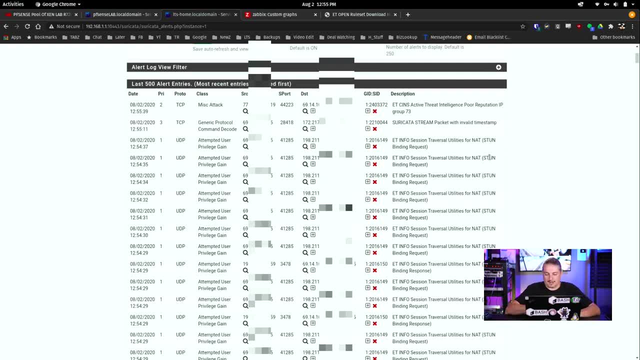 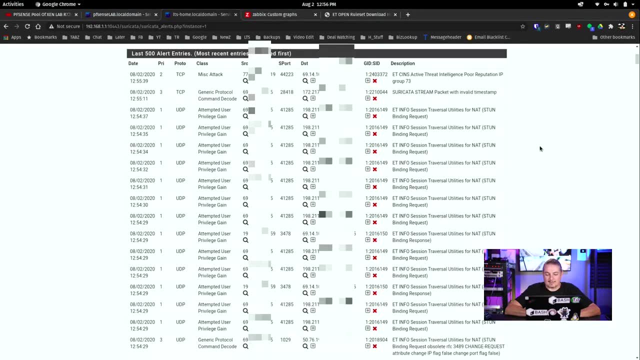 be uh, doing some torrenting. uh, you know, seeding some isos for open source downloads and things like that. so we definitely see a lot of that inside of here. so e you know, you get the stun protocol. that is actually not for torrenting. that is from let. 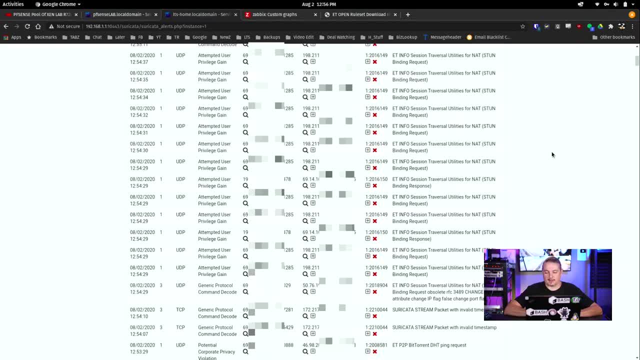 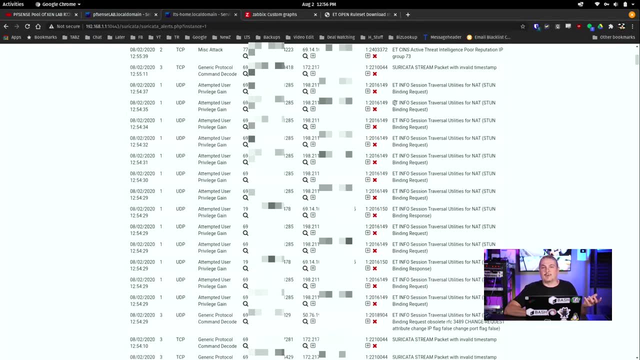 me look: sync thing server that i have running behind there. it actually uses the nat traversal with stun to contact out. so once again we have an info session. and do i care about this? do i know it's a false positive? yeah, because i looked up what it was. so how do we get rid of that rule? 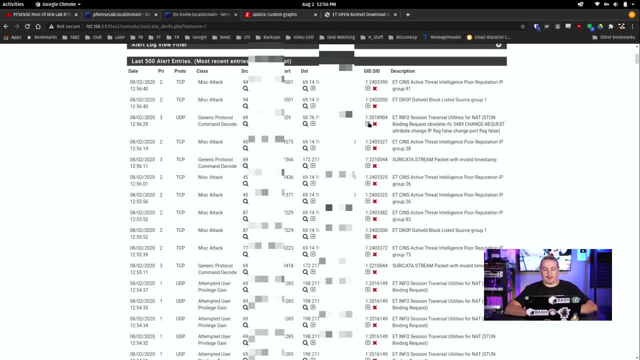 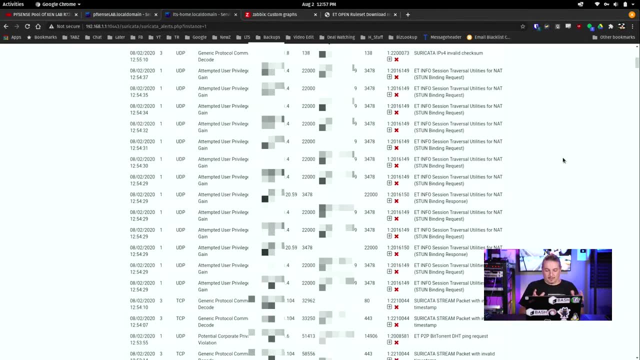 and how do we get rid of the annoyance of it being on there now? by the way, i'm going to switch over real quick to the land side. we're going to see those same coming up again. so from- and i know i'm blurring the ip addresses so you can't see this- 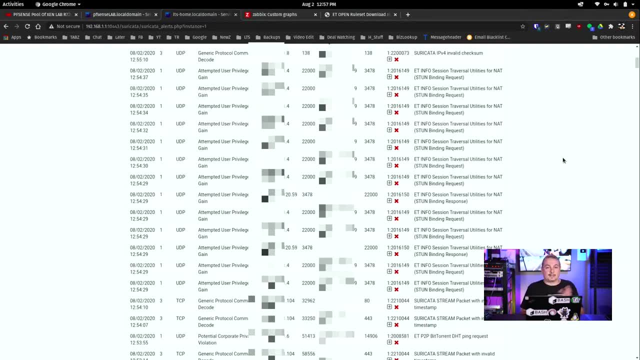 when you do it from the land side, i get the internal ip address. when i did it from the wan side, all i get is the wan ip address and where it's destination to its other public ip, making it a little bit less useful. when i look at this rule, though, from the 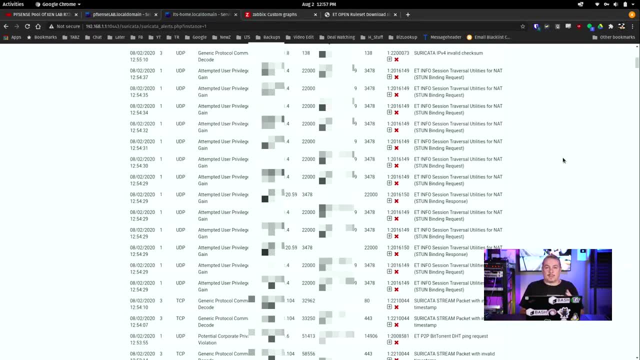 land side. it's easy for me to identify because i know what that particular ip address internally runs, so i can go: oh, i know that's running sync thing. i know that server is reaching out to. is the sync thing stun server for nat traversal? so i know it's good and i know internally. but 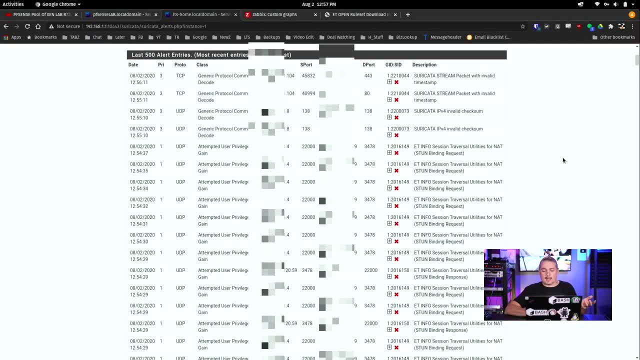 by having that on there on the land, on the land side, like i said, much more effective. you have it on the wan side. all i know is the public ip address, which i already knew. it's my wan address and the other public ip address where it's going to, but that's not telling me what server behind. 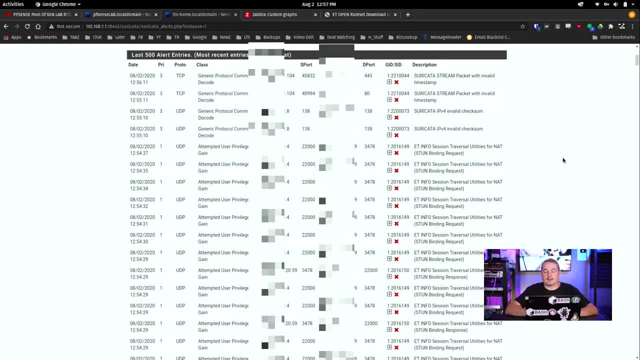 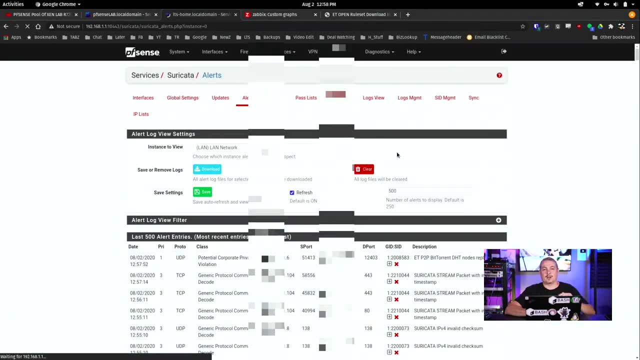 my firewall did it. that's one of the other reasons that's important to have this on the land at the wan. but now we can talk about getting rid of this rule, and we've done no tuning in the rules. i just turned them all on. select all said yes, so we're going to go over here and we'll get rid of this. 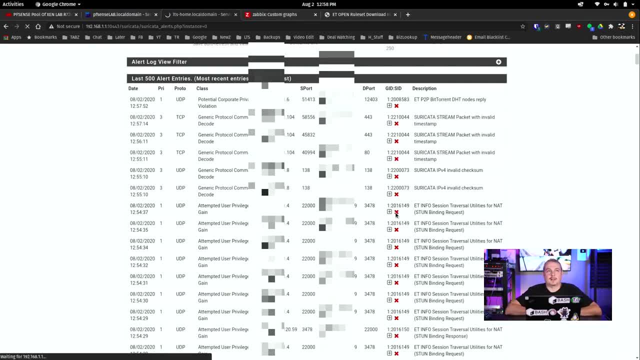 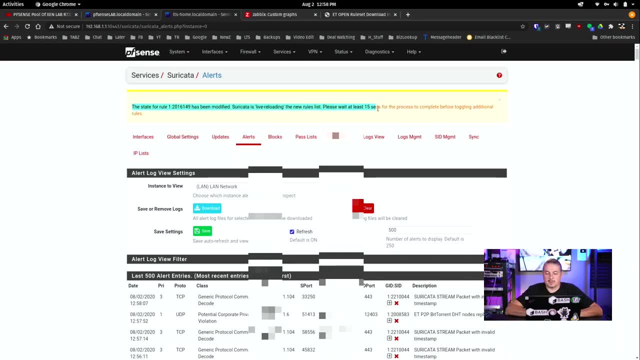 rule right here. please click it. it spins for a second. all right, the state of rule has been modified. seracada live reloading with new rules. please wait 15 seconds for the process to complete before toggling additional rules. this is important, and how long it takes really depends on how fast. 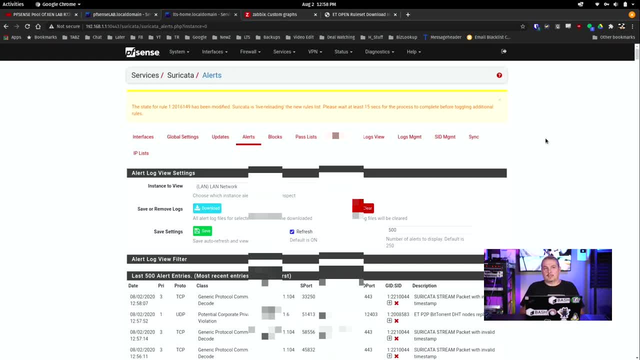 the system is, but for each rule you disable you need to give the system time to reload the rule set before you start doing more of them, or you can have the system well. i think i've seen seracada crash if you try to do it real fast or just get stuck and not properly reload rule sets. 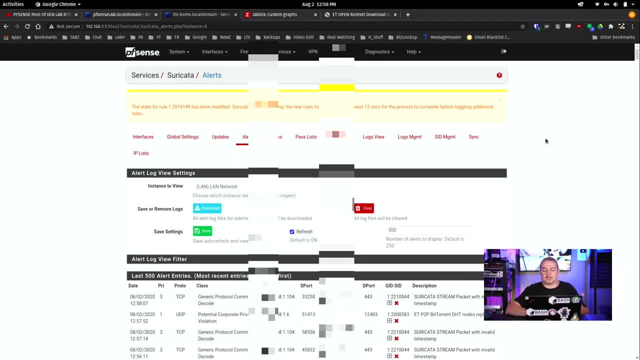 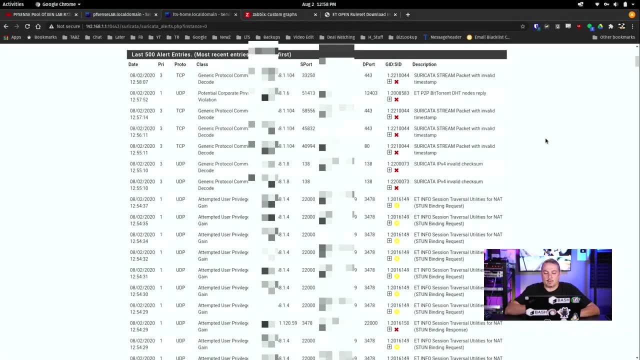 so give it a second for each one you disable. depending on the speed of the machine, not a big deal. so now you see, all these are yellow. what that means is they're not going to show up again, but they're now in the log history that they were there. 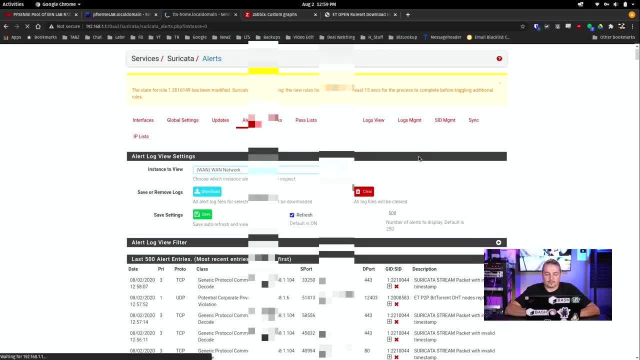 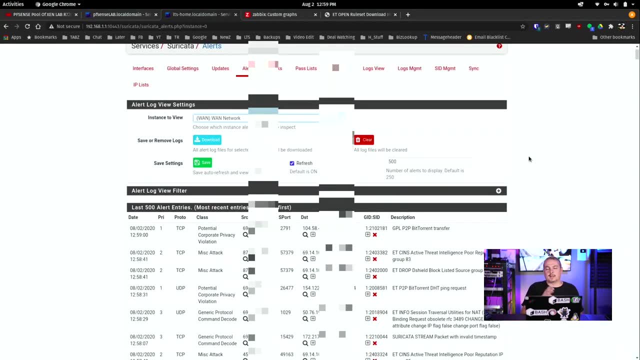 so this is on the land side. let's switch over to wan. they're not yellow and the reason they're not yellow here is because all rule tuning is on a per interface. this is why one of the advantages: if you take the time to tune one interface and then clone it, all those rule changes you made and all those suppressions you 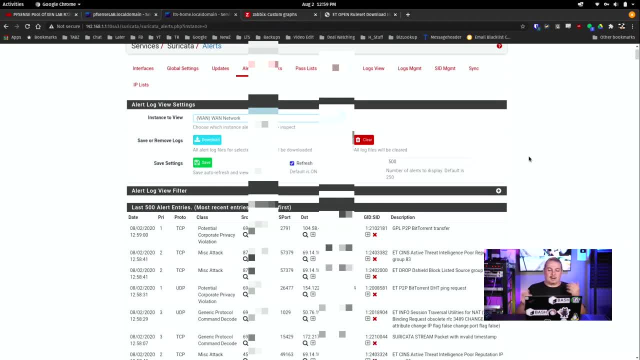 did will follow that interface clone. if not, if i want to, if i have the same problem repeating on multiple interfaces, well, i'm going to need to go through here and tune it on each into interface and keep going through, and keep going through. also, this is one of the reasons i mentioned. 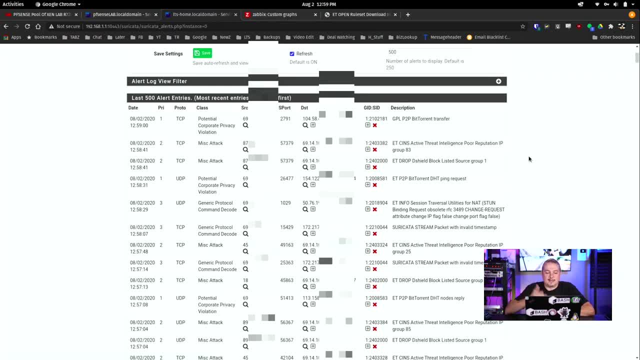 blocking can be really bad, because if i had blocking turned on and these things have a method by which they want to say block and it's part of the rule set. so some rules are just notices, but some rules are like: all right, this is something bad and we're. 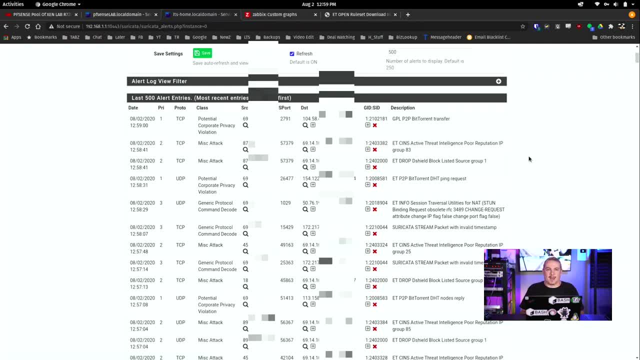 going to block this ip address. well, when you start blocking everything now, you have the problem of sorting out what broke, why certain things don't work, and especially if they're in a shared hosting provider where something else may reside. that's where those false positives and can really create. 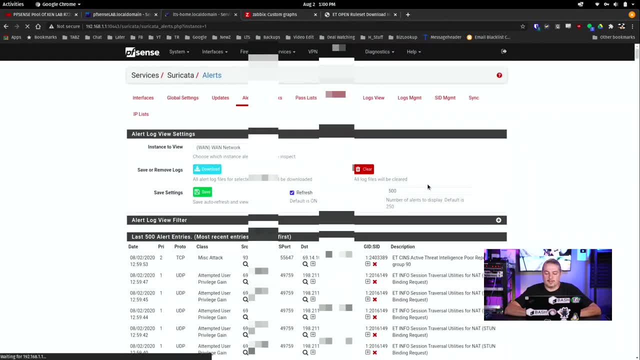 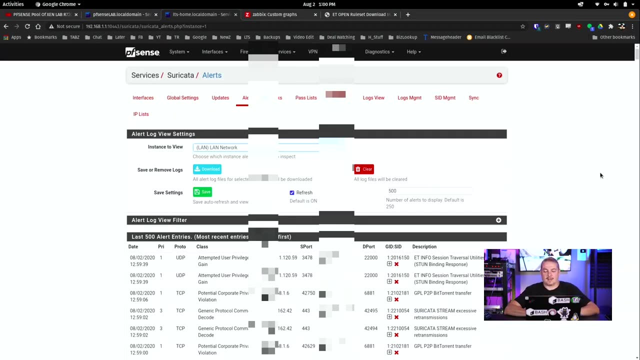 a headache and a blocking. so tune the rules first. now other things that are maybe less obvious. let's go back over to the land side again and, by the way, this auto refreshes, um, while you're watching this, so the default is auto refresh on as you change it to like 500 to show me 500 of the logs. 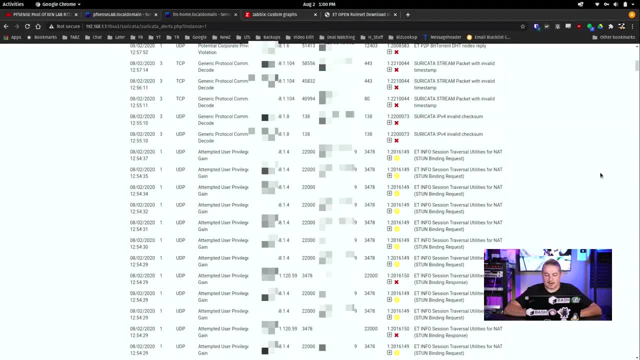 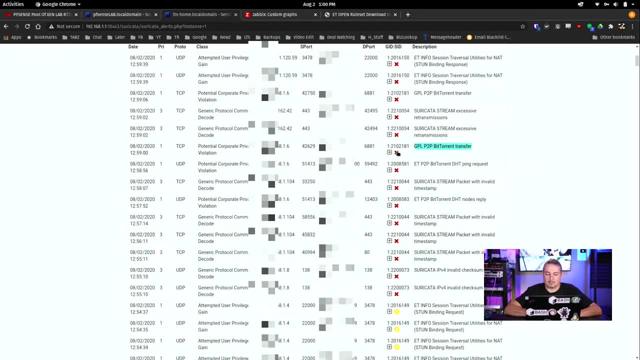 here when it goes. so it's always got plenty of information in here. so let's see what else? do we have gplp to be bit torn transfer- well, i know that is definitely what's going on there, so we're going to head and clear that one. all right, now that rule is cleared. what other rules do we need to clear? so 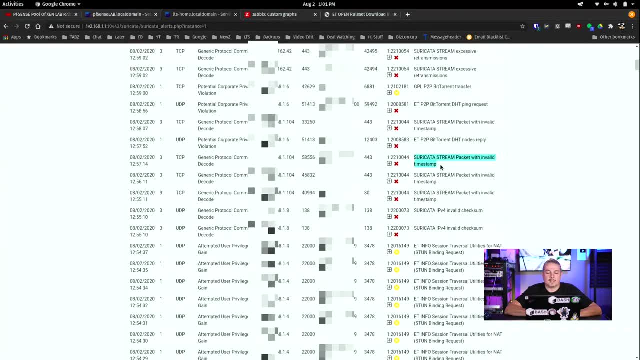 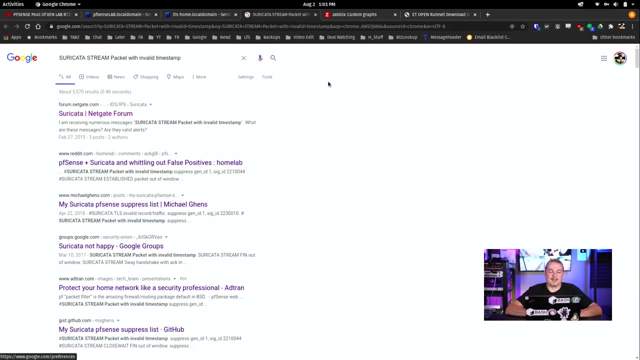 siracata stream invalid timestamp. now, these can be tricky, it's more of an annoyance- and right-click copy or paste into google or, if you're using um, so you can do it like this in chrome: search google for siracata packet timestamp and look we land right here on the netgate forum where apparently 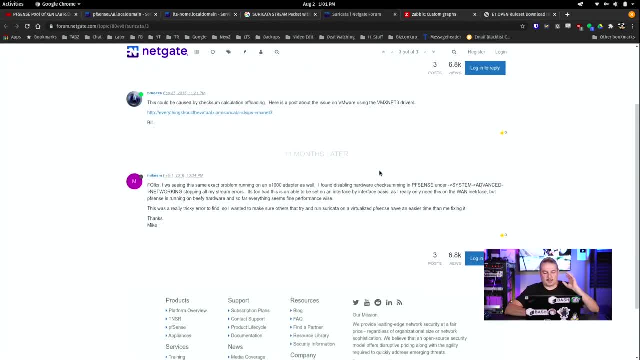 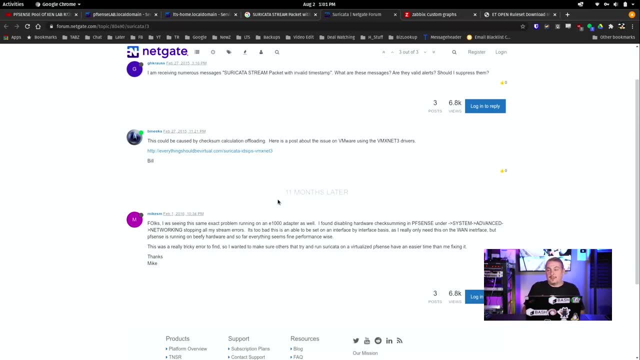 and i've already seen this one enough that i know what it is. there's a problem with certain stream errors based on certain interfaces having this issue. now, this is a problem that we're going to. this is where you're going to spend a lot of time and you're going to get an idea what they actually 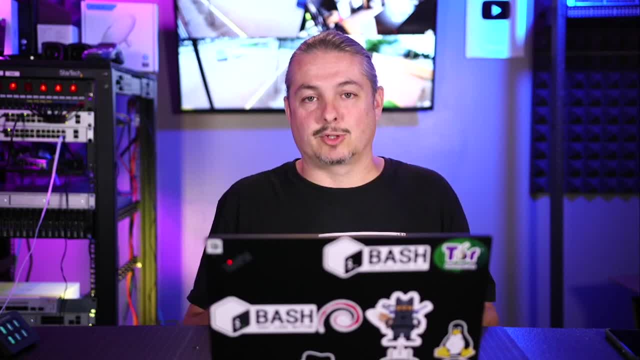 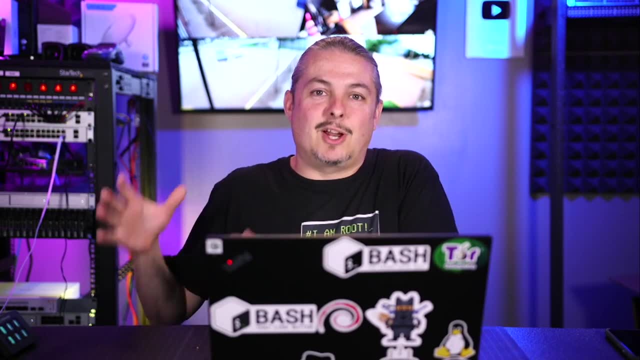 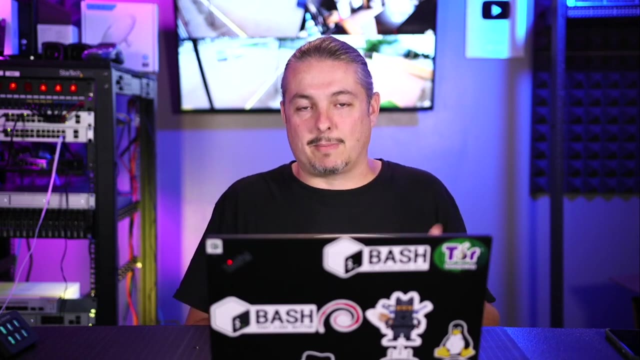 do at these network operation centers and why, when you buy a commercial firewall, this is a paid service to have intrusion detection, intrusion prevention, properly working and set up. there is a team of engineers that spend a lot of time looking at all these errors, figuring out whether or not they're false positives and sending that data back and forth down the pipe. this is 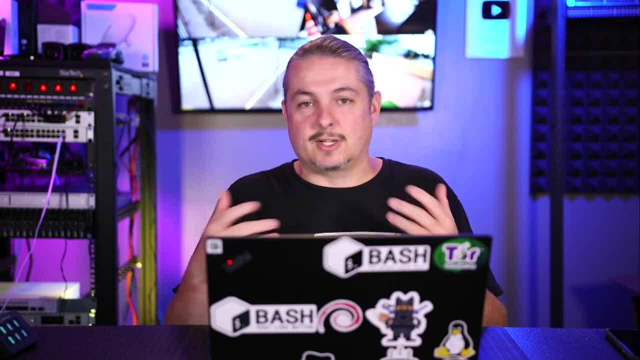 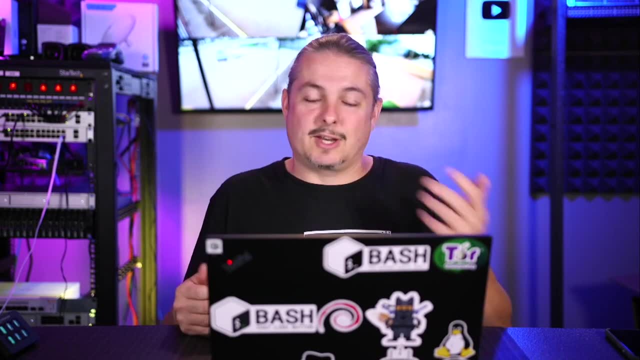 essentially what they do with a network engineering center, security operations center. you're going to find them going through looking at all these, determining whether or not it's going to be a real threat or just another piece of noise in the system, and deciding whether or not that needs to. 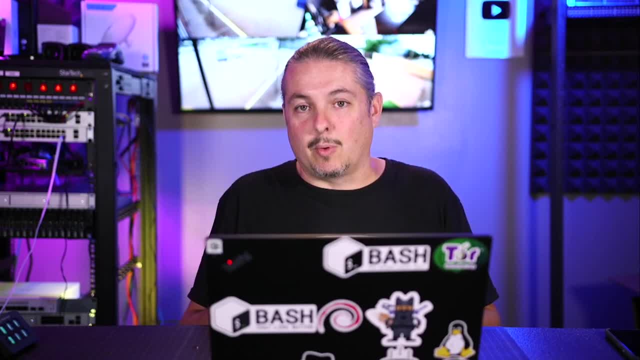 be stopped and, you know, flagged as get rid of that rule. this is why it's not a set it and forget it type system. it is very important to understand that's what these engineers do. that's what you're paying for when you buy a firewall with a subscription service to an intrusion prevention. 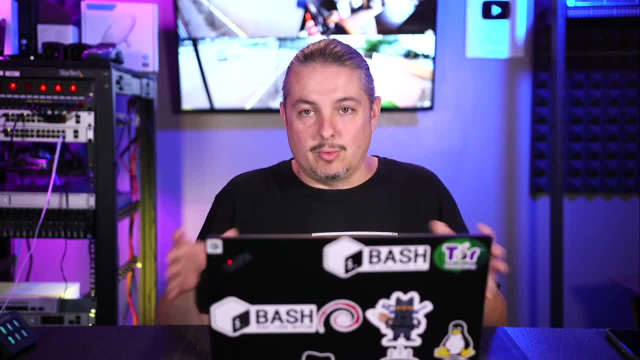 system on it and you're getting a more honed fee that they're looking at these and going through it and going all right. we see this rule, we see this many people doing it. we realize it's. they will dive deeper, maybe doing a pcap on it and go all right. that is definitely not bad traffic. so 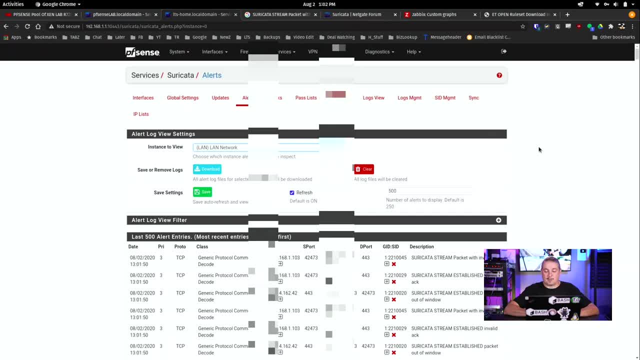 just some notes on. when you're looking at these, you do have to spend some time going back and forth to do this and going through figuring out which ones are real, which ones are not. so there's actually quite a few of them in here for this, uh, invalid ac. so let's go ahead and 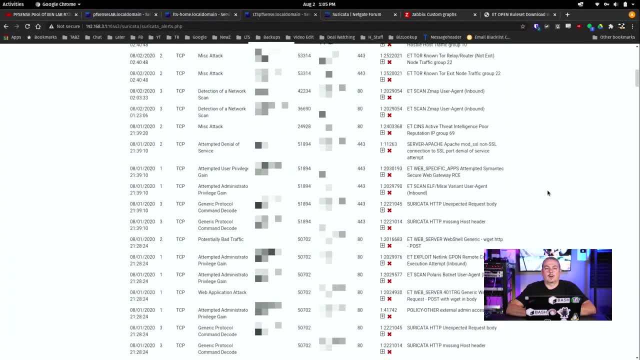 uh, suppress that one, i don't need it all, right? so here we're going to jump over to another system. i have running siricata, which is our system here, and because we host some web servers, we get some interesting things, because, well, people like to bang away at. 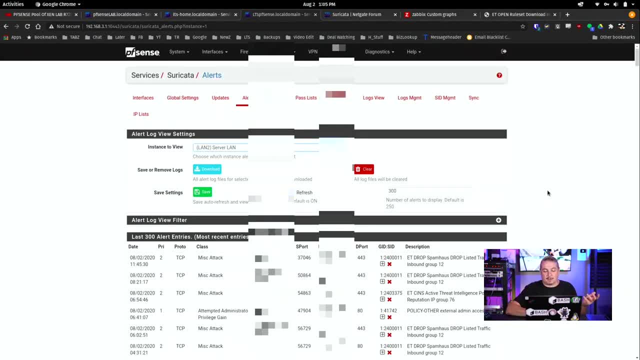 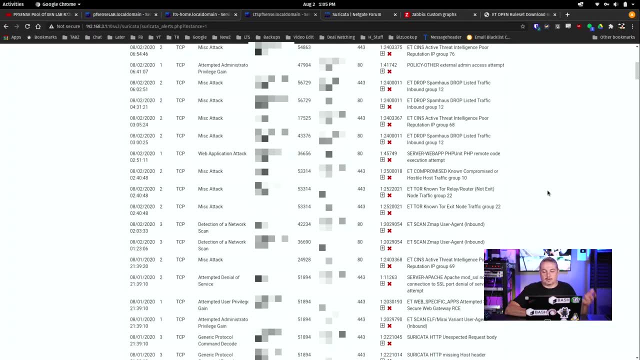 them and try to figure out how they can get in, which does get a lot of these people blocked all the time. so this is specifically a network dedicated to where my servers are that run things like host my web services that we have public facing and it's interesting to. 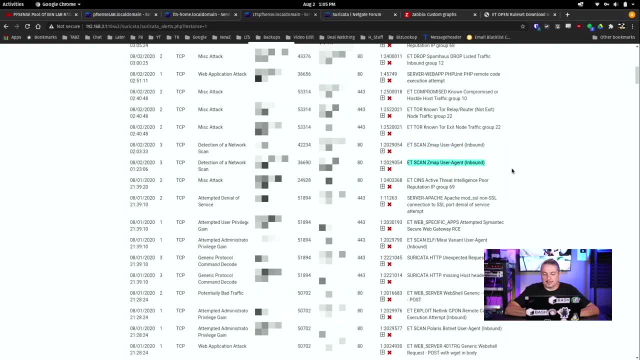 see just how many scans. and we do block the people who scan us. so you scan us a few times, you're done, you're blocked for a long period of time. then we have the poor intelligence, poor ip reputations. those are in here as well. uh, specific attempts: someone tried to attempt and these are: 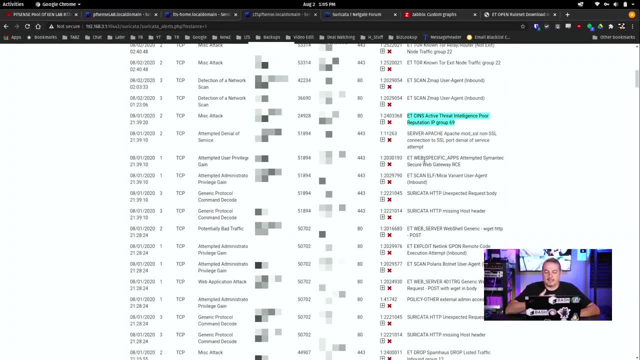 all those essentially false positives. in some way they tried something that doesn't exist. so this is web specific apps: attempted semantics secure web gateway, rce. this is what gets. really interesting is the. this is a remote code execution against the semantics secure web gateway, and this is what you'll end up seeing a lot of if you have portso. 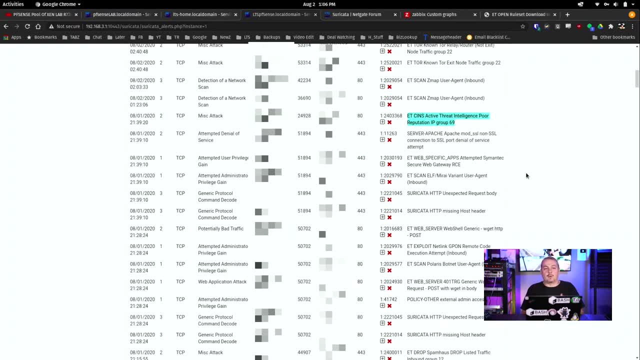 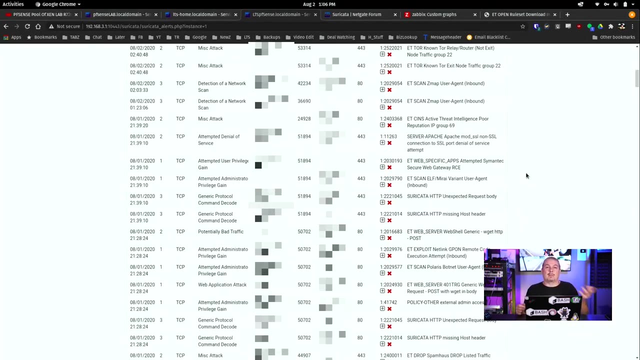 in where siricata has an incoming piece of noise that it detects going. all right, someone tried. we recognize this attack pattern. this is a semantic gateway endpoint exploit. you know remote code execution, that they tried against this but failed because one i don't have one, but siricata blocked. 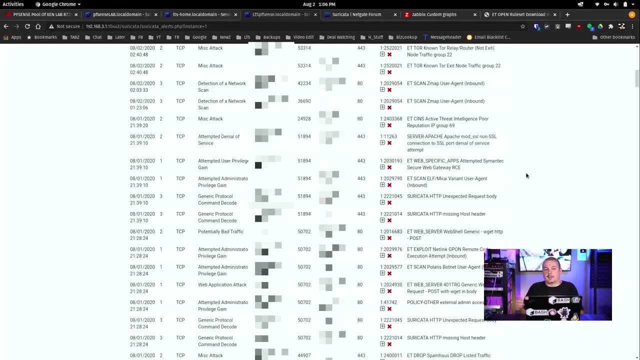 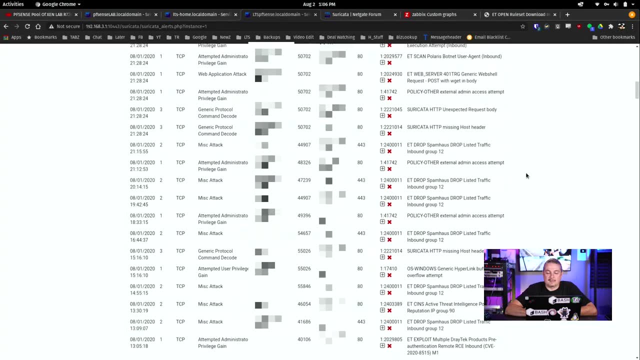 them anyways, because if they're going to try that, they're going to try other things. so these are botnets just hammering away. so this is where siricata, to me, is a little bit- well, i should say a lot- more effective, because it's blocking these kinds of things that we're going to be able to. 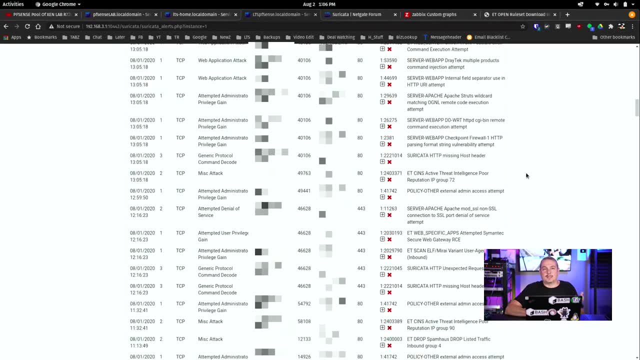 run constantly and looking for these type of threats. now, even though these don't apply to me, what if something did? what if there was some flaw? an apache server and i'm running an apache server, or an nginx server and i'm running an nginx server and it detects that attack. this is where siricata. 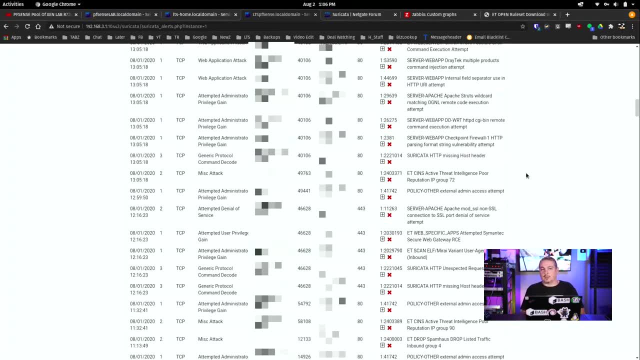 can be very effective and, to me, much more valuable than trying to monitor iot devices at my house or, you know, dealing with false information that it gives about the syncing tool that i have running going. oh look, we found this or found that, because, so one, eventually, there wasn't too many in there. 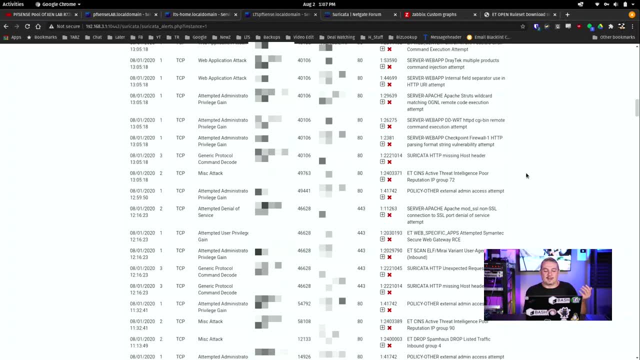 since running it this morning at my house. there wasn't too many false positives on there, but, um, they do happen from time to time. but when it comes to running it on my server side network, that's where we have the most luck with it, i should say, or the most effective use of it, because 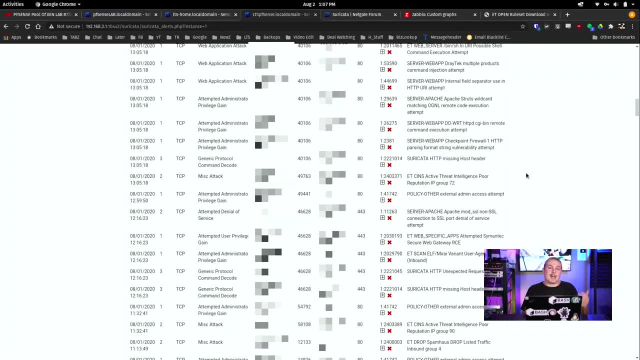 it goes through, it sees things that are potential attacks, and if a bot or an ip address is attacking you, you know once, then it's probably attacking you in other ways. if it finds it, even though there's no response, as in the rce against the semantic gateway, because i don't have one. 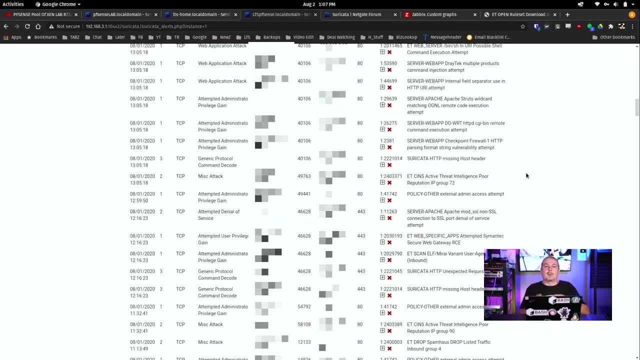 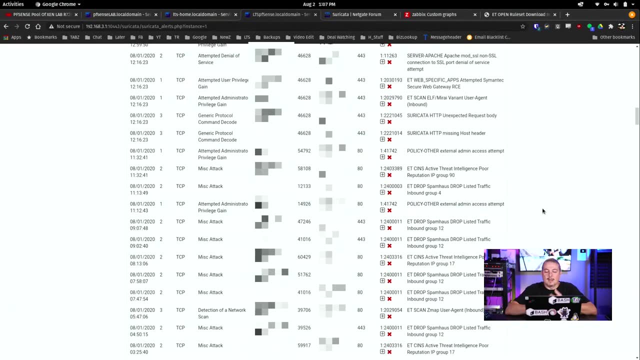 it goes. what else is on there? it answered. so let me try again. well, by siricata blocking it, it blocks any further answers because that ip address just ends up in a block list on here and keeps them from scanning further. so this is where i think it's a lot better. 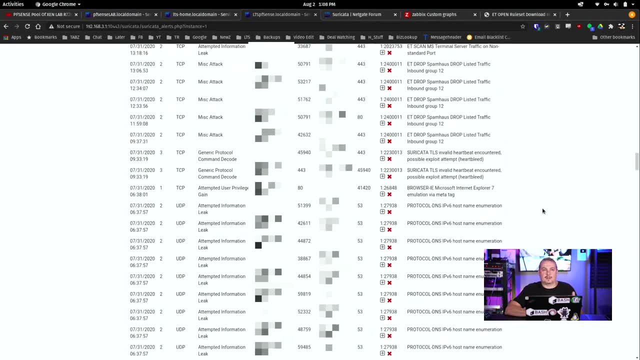 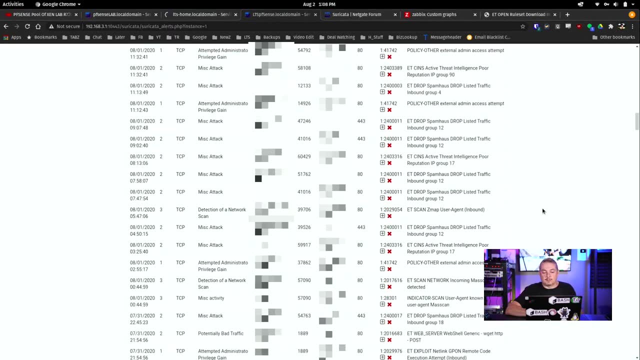 but, like i said, it's only limited because it still can't see into encrypted traffic. it just has to match these and we're still dealing with false positives on tools we use. so it's something we have to kind of be, you know, actively monitoring. now the last thing i want to talk about is the 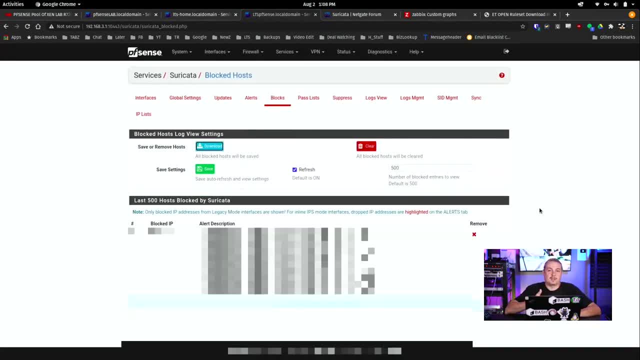 last thing i'll show you is the block list themselves. so that checkbox i mentioned where it turns on blocking. you can turn on blocking and you can go through and get rid of blocks if you want, because if they're false, just get rid of them here. if not, maybe you want to leave them here and 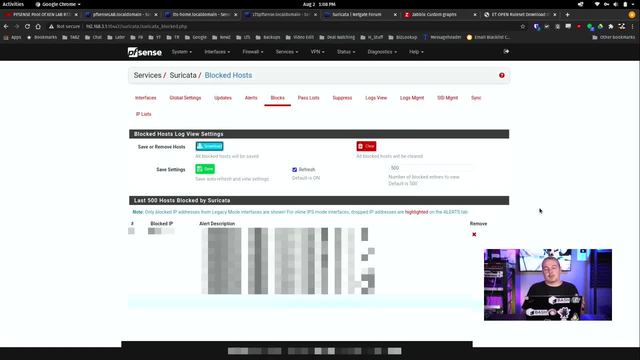 then, as i stated earlier in a setup for the default amount of time you want to have those blocks on there. that's kind of an up to you. so maybe you want those blocks to last essentially forever, not forever. that is a up to you tuning portion of this to figure out how long you want to keep those. 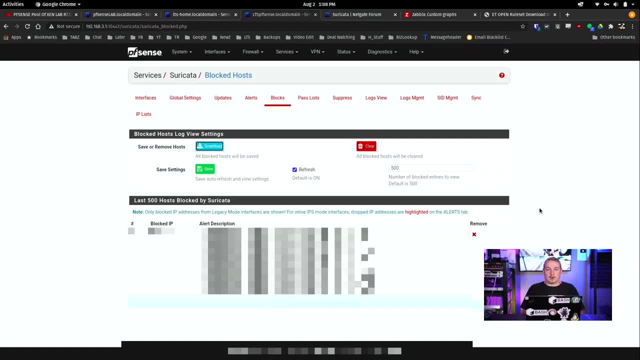 things blocked for. but fair warning: sometimes, due to shared hosting services, you may find something that gets blocked even by false, but then all of a sudden everything can't get to it. now, the way it blocks inside a pf sense if this ip address gets blocked even though it was blocked on a separate network, such as my.